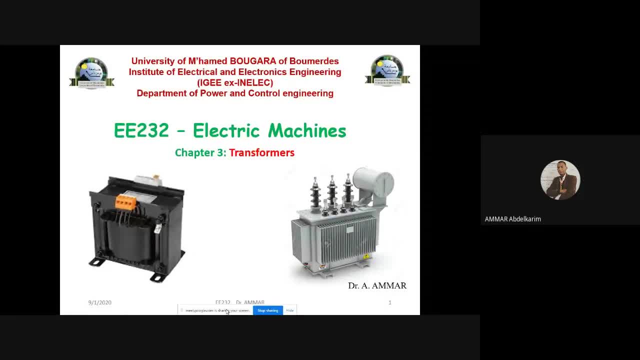 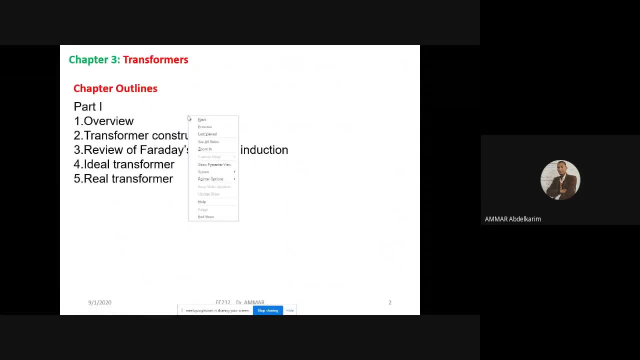 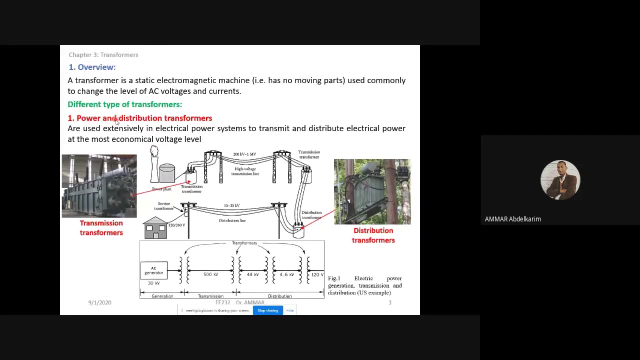 Our electric machine is the transformer. okay, So the outlines of this part are: overview: transformer construction, review of Faraday's law and induction ideal transformer. and the last element in this part is the real transformer. So overview. a transformer is a static electromagnetic machine, So the transformer is an electric machine. We said that the electric machines that are devices that transform the form of energy from electrical to mechanical or from mechanical to electrical. 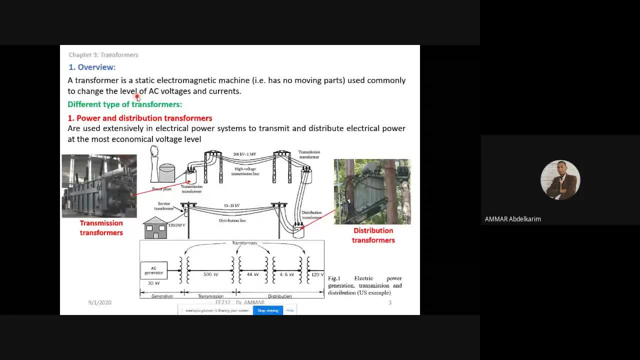 But the transformer is a static machine. We don't have motion, We don't have rotation. So this static electric machine transforms the form of energy. It transforms the electric energy from electric form to electric form with different amounts of voltage and currents. So a transformer is a static electromagnetic machine. It has no moving parts, We don't have a rotor. 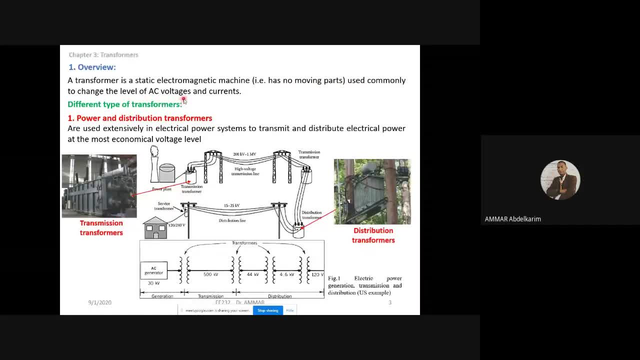 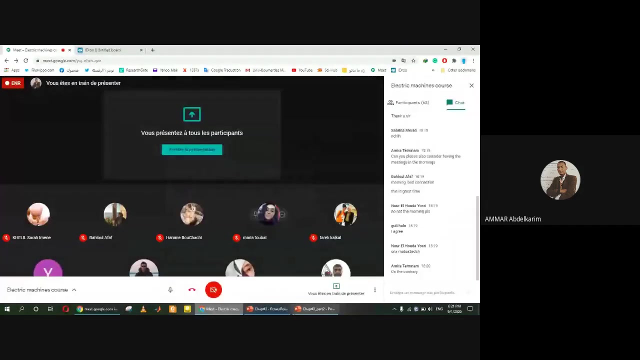 We use it commonly to change the level of AC voltages and currents. Okay, Different types of the transformer. We have, of course, different type Of transformers, So different type of the transformer. The transformers we care a lot, of course, are the power transformer of distribution and transmission. 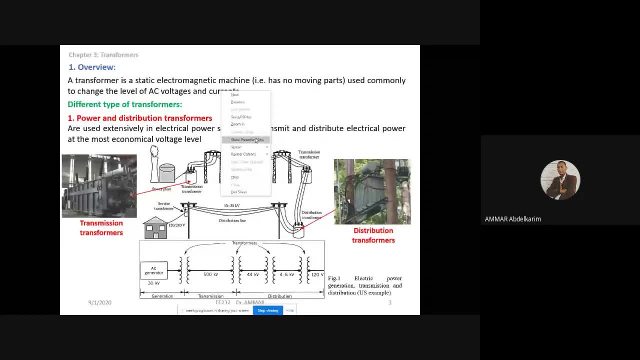 So I show you before, in our first session, a picture like this which is different phases: How the electric energy, How the electric energy. So I show you before, in our first session, a picture like this which is different phases: How the electric energy. 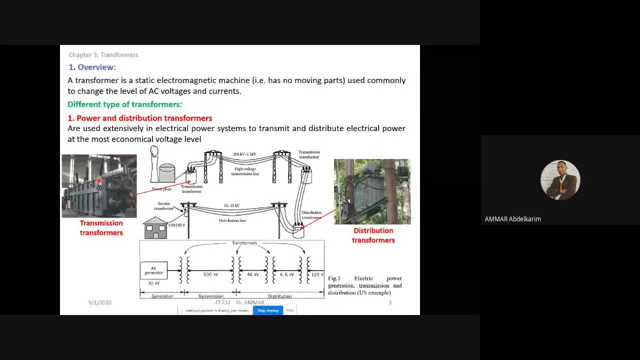 How the electric energy. So this here here we see a bar plant where the generic generation done, So at the output of generator we have to rise the level off the voltage And I told you before this is a for economical reasons. When we rise the level of the voltage using those, we call them transmission transformers. when we raise the level of voltage, the current gets decreased, And when we decrease the current, the cross-section of the cables that use it for transmitting the energy gets reduced also. so this is for economical reasons. So then the electric energy is transferred through those transmission lines. 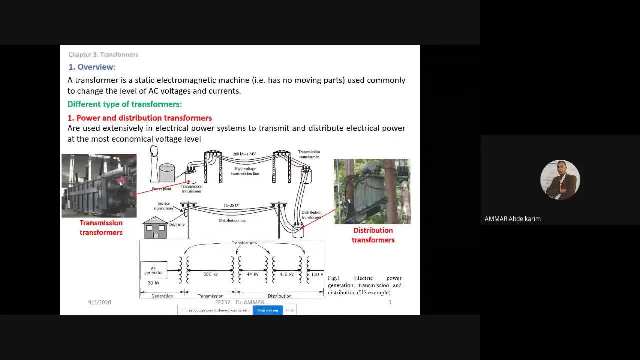 Then from transmission lines we have transmission transformers. you are seeing them here in the figure. After the transmission transformers, those are used here, for example, to interconnect different networks with each other. So you may find transmission transformers not in the power plant, but we call them substations. 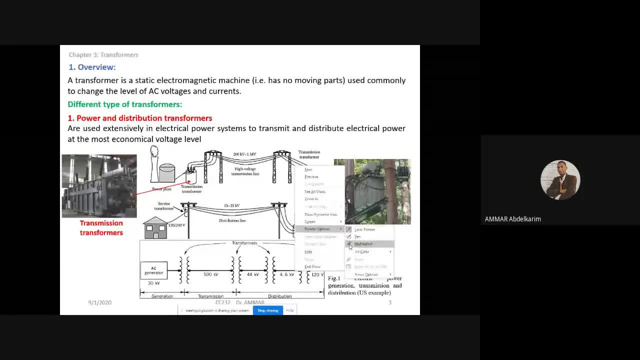 here We call them substations, those stars. here. Those substations are used to connect the networks between each other. After the transmission transformers we have distribution transformers, So those two reduce again the level of the voltage. You see this example. the level of the voltage here is between 200 kilovolt and 1 megavolt. 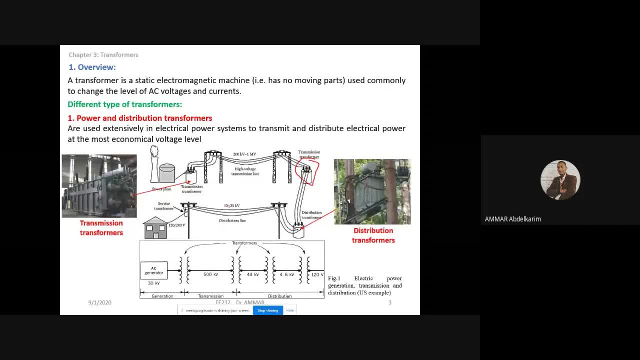 and the level of the current, here of the voltage. here The value of the voltage is between 15 and 25 kilovolt. This is the example. of course it's not for our countries. We may, here in Algeria, we may, find different levels of the voltage and the currents. 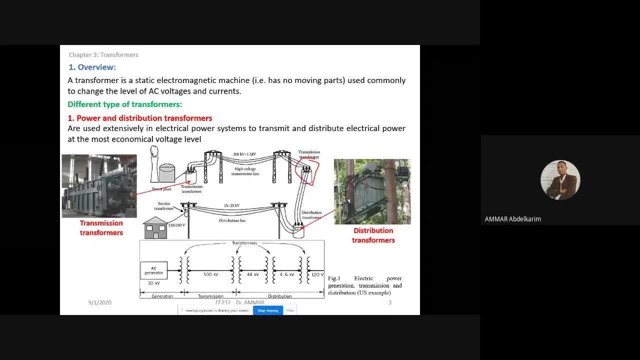 After that we will have service transformers that transfer the electric energy to the consumers, And the figure below concludes this cycle. This is an example of the US, of course, AC generator. The level of the voltage here: 30 kilovolts. 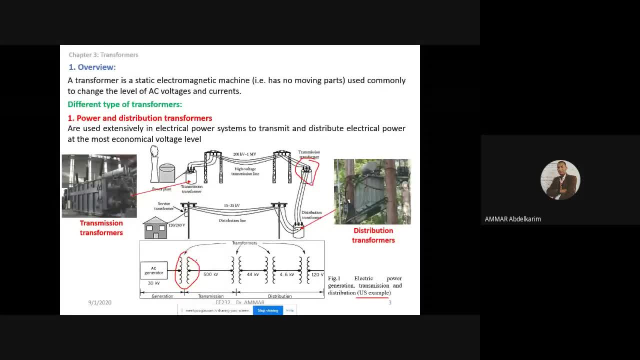 So the transmission transformer will rise this voltage into 500 kilovolt, Then the distribution transformer. they have different levels, So the first one will reduce the level of the voltage from 500 kilovolt, Then the distribution transformer. they have different levels. 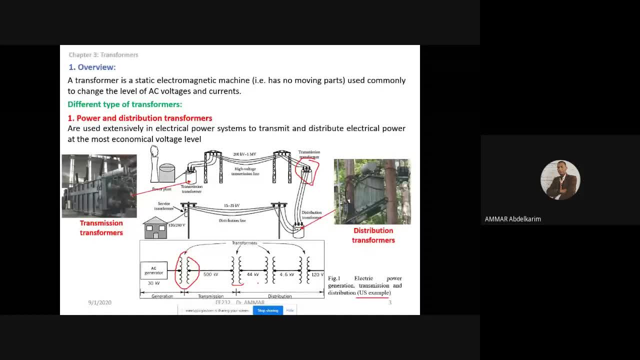 The second one rises the voltage from 5 kilovolt to 44 kilovolts, Then 4.6 kilovolts, Then to 120 volts, which is the service electricity that is used in houses and cities. Okay, 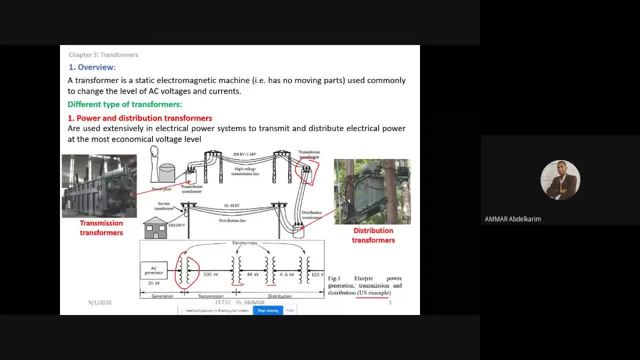 So this is an example of the US power generation, transmission and distribution. And this is just to show you the importance of the transformers. Okay, AC network. so we cannot make an AC network without transformers. Let's move to the next slide. 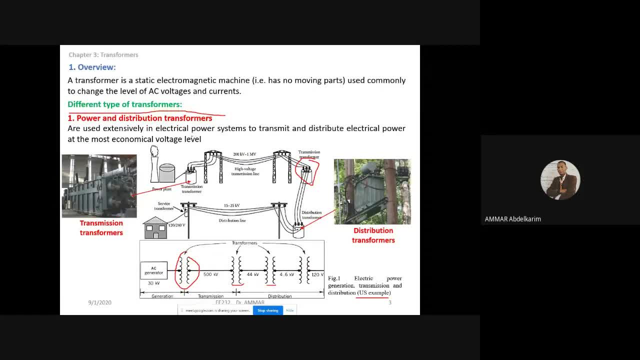 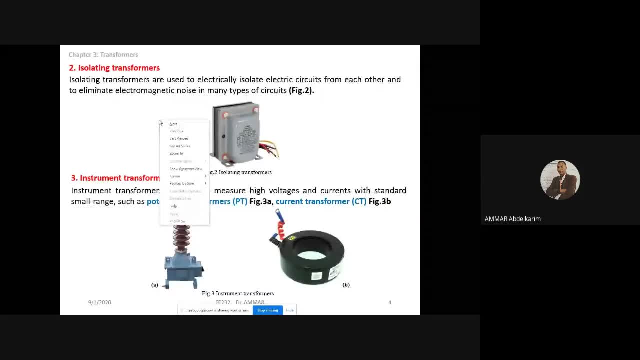 So this was the first different type of transformer, which is power and distribution transformer. The second type of the transformer, let's use a different color. The second type is isolating transformer. So this isolating transformer we may found it in some electric installation. 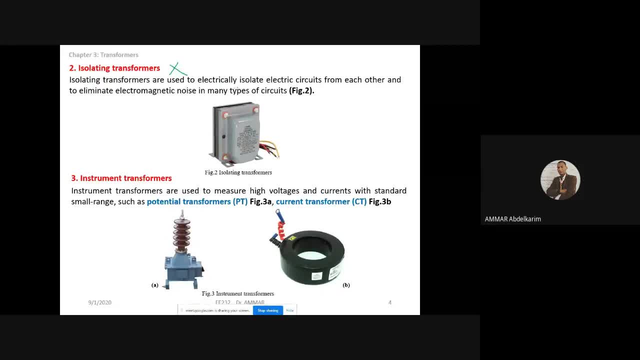 Isolating transformer are used to electrically isolate electric circuits from each other and eliminate electromagnetic noise in many type of the circuit. So this type of transformers. It does not increase or decrease the level of the electric energy, So its input, the voltage of the input, equals to the voltage of the output. 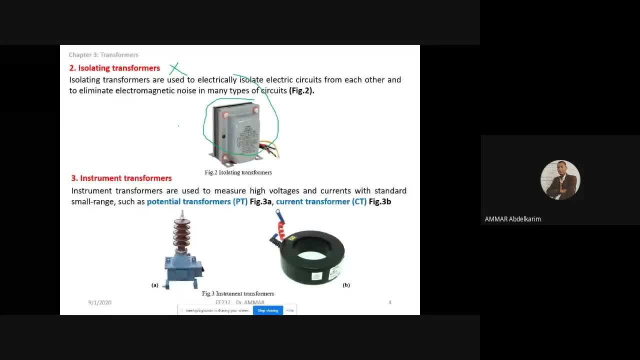 Also, the current of the input is equal to the current of the output. These transformers are placed in such electric installation just to provide a physical isolation between two circuits in order to eliminate such noise. Okay, So these transformers are placed, or can be used, also for a protection purpose. 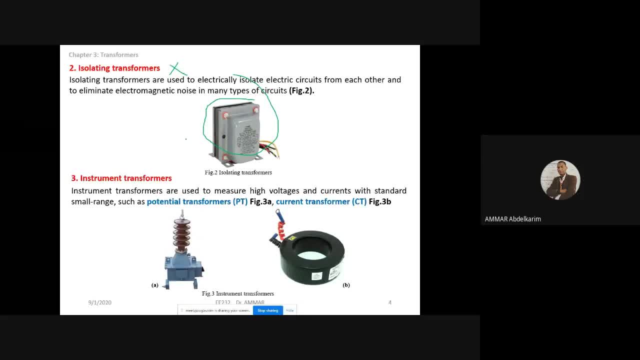 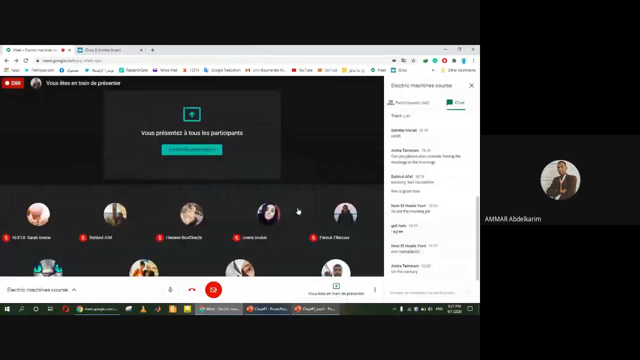 In such electric circuits or in electric installation. we use those transformers. They don't increase or decrease the level of the voltage of the current. The input is equal. their inputs is equal to the output, But they use it to provide that physical isolation. 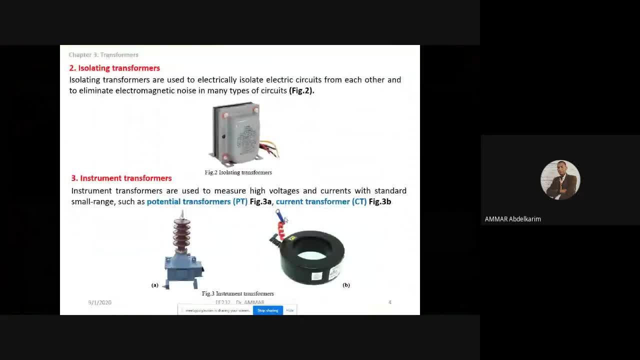 Okay, So this is the separation between the circuit elements. And the last type here is the instrument transformer. So those transformers are used for measurement. For measurement purpose We may found a potential transformer like the one shown here, And these also used in the networks because we cannot measure the high voltage directly. 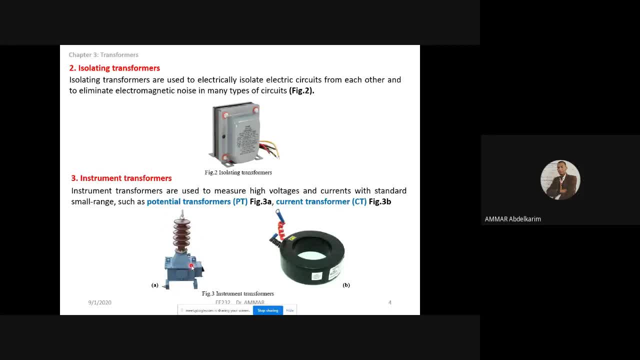 So we use those potential transformers And also we call this a current transformer. The instrument transformers are used to measure high voltage and the current with the standard small range. So those transformers of the current or the voltage use it to measure the high voltage and the high current. 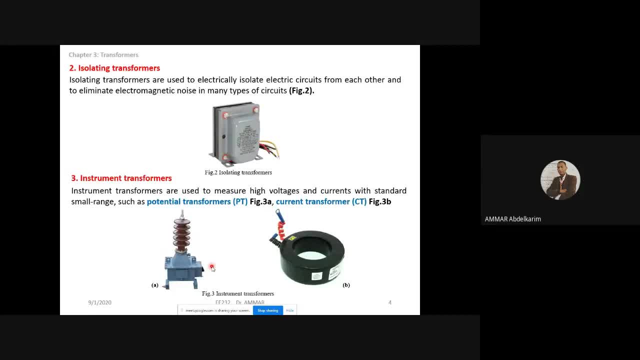 So those devices give us? They have what we call a coefficient or a factor. Okay, Okay, The piezoelectricity. The piezoelectricity, A factor, indicates to a higher voltage. They may be, They may divide the voltage over 1000, for example, or just they have ratio of a report. 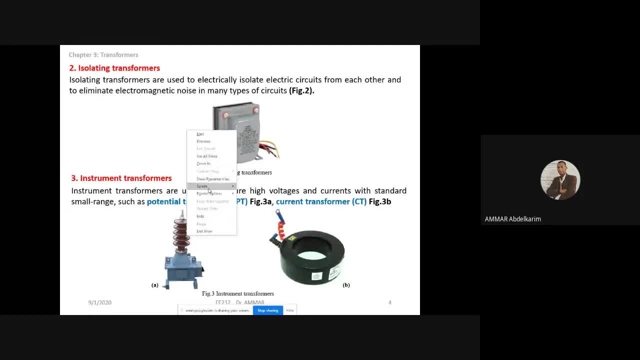 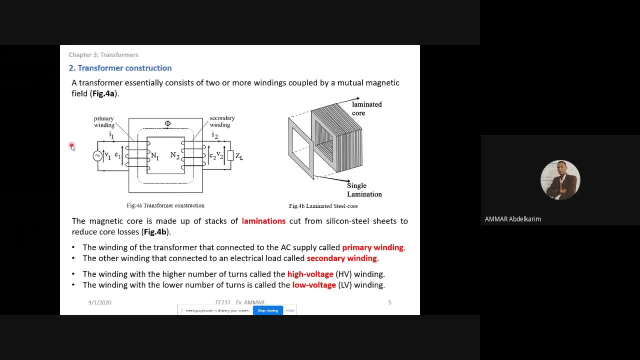 to give us to indicate the real voltage value. So those are the types of the transformers: Firstly, the power and distribution transformer, The second one is the isolation transformer And the third one is the instrument transformer. Okay, transformer. now let's see the construction of the transformer, of course, 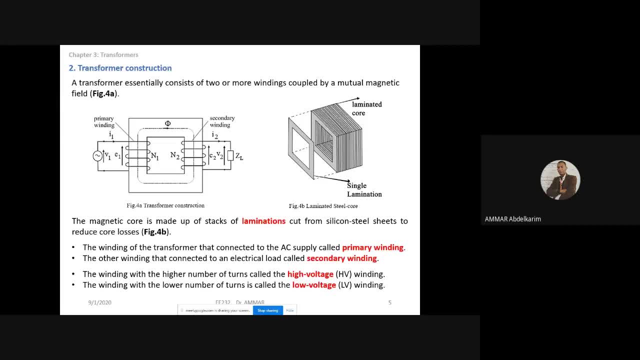 the transformer is a magnetic circuit. the transformer is essentially consisted of two or more winding coupled by mutual magnetic field. mutual which means mutual, it's between them. so the flux here in the core is the flux of both coils or windings. okay, so the transformer essentially consists of two or more winding, more maybe in the three phase. 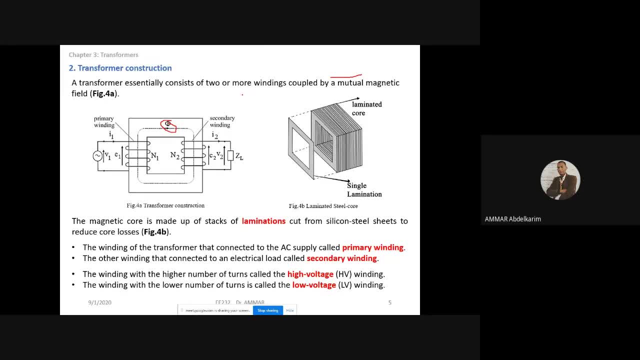 there is also three phase transformer, but here we are going to focus on the single phase transformer- coupled by mutual magnetic field. so the magnetic core is made up of stacks of laminar, so lamination, which means sheets, thin sheets like as you see here in this figure. those are the sheets compacted with each other to consist the core. so 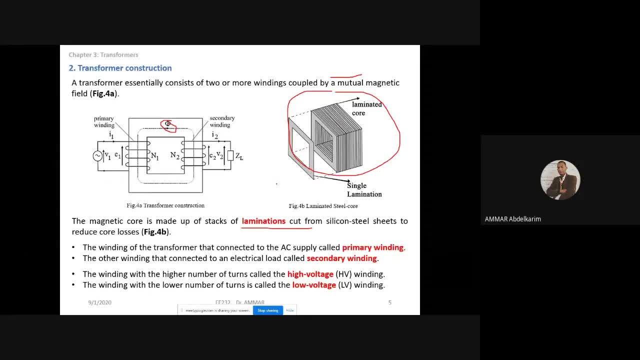 this is a single lamination and we so we know what, why we use those lamination: in order to reduce the eddy currents in the core. so this is the construction of the transformer is constructed by a core made from lamination, from silicon steel material- here is silicon steel- to reduce the core losses, exactly, which are a 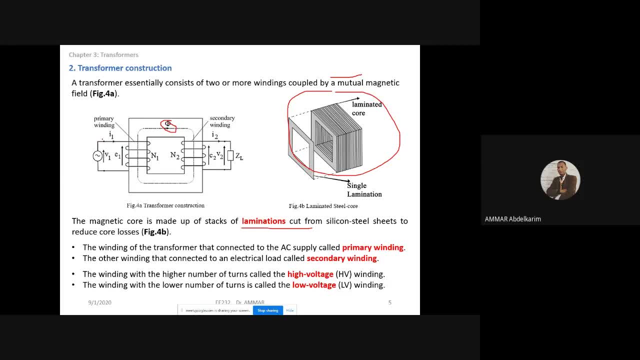 occurrence and we have to wine this, the first one in the 놀�aph свои 1989 and the second one we call it secondary guidance, and the winding of the transformer that's connected to the AC supply, the winding that's connected to the source, called primary winding, and the winding connected to the load, called secondary. 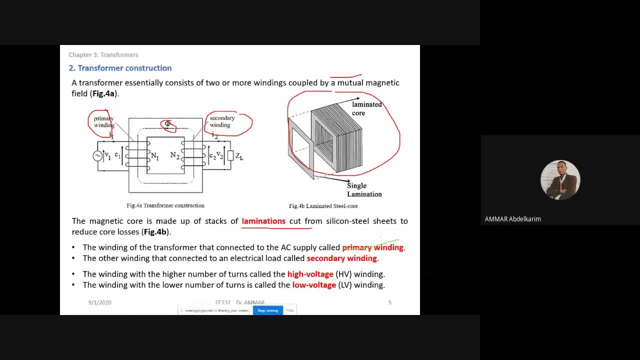 winding, So we can call them primary winding and the secondary winding, and we can call them with other nomination: The winding with higher number of turns called a high voltage winding, HV, and the winding with lower number of turns called low voltage winding. 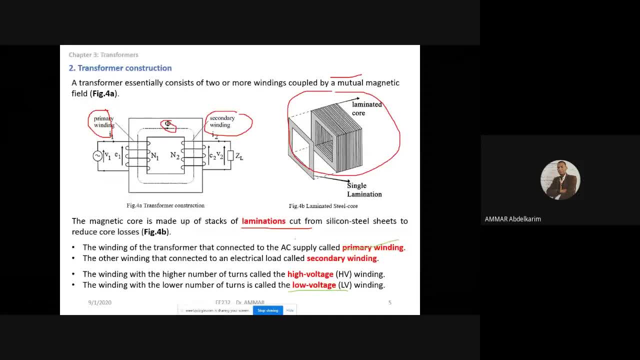 So here the high voltage winding can be primary and can be secondary. Also the low voltage winding. it can be primary and can be secondary because we have a step up and step down transformer, The transformer that rises the level of the voltage and reduces the level of the current. 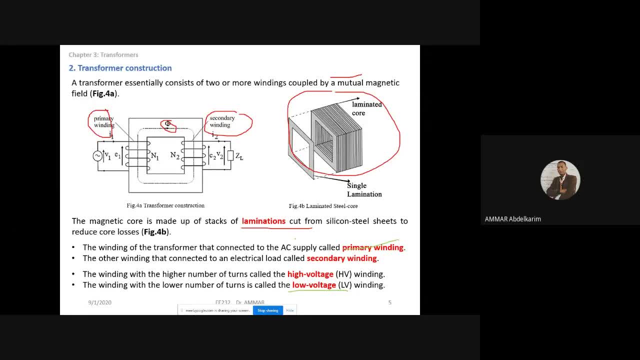 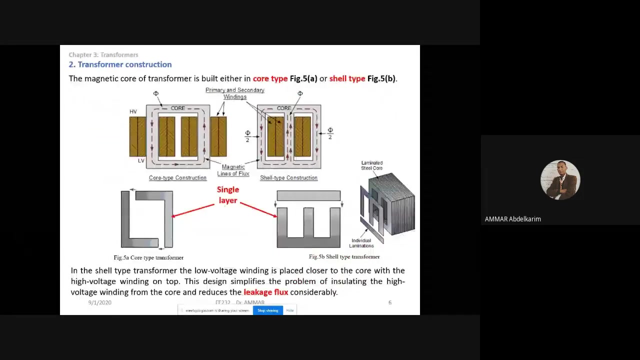 and the transformer that reduces the voltage, And the same transformer can be used for both purposes. If we choose the first one, the high voltage as primary, it depends if we choose which winding is: the high voltage or the low voltage. Let's move to the next slide. 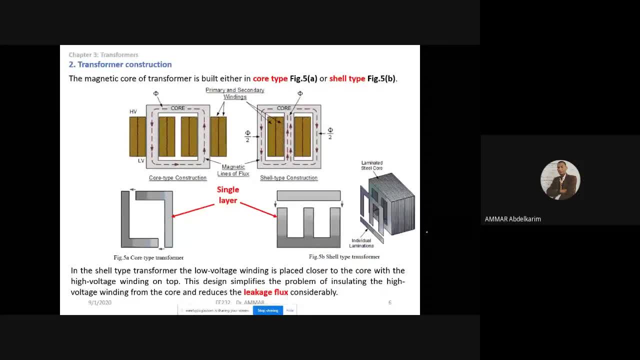 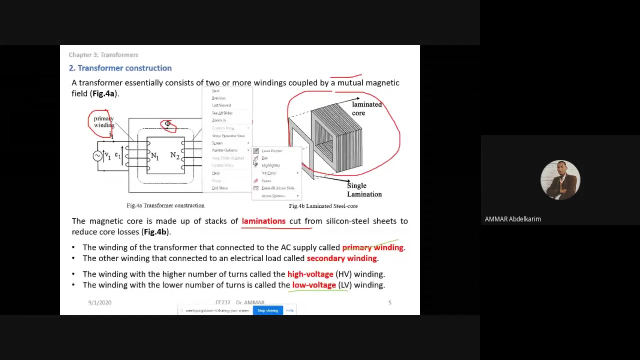 So we are also with the current In the construction. we may find two different types of construction. This is the simple one, which is called a core type. as you have seen in the previous slide, This construction is called a core type, a core type transformer. 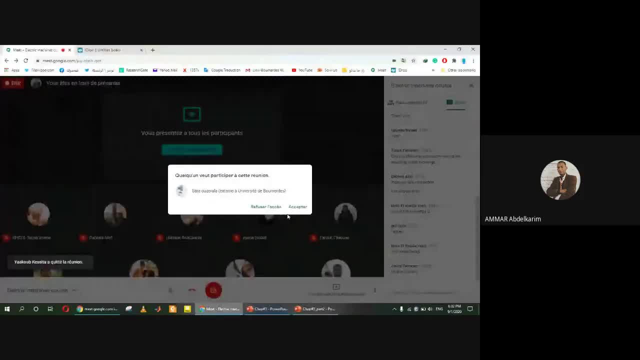 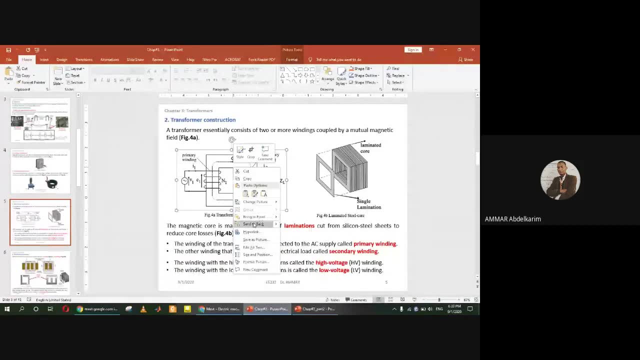 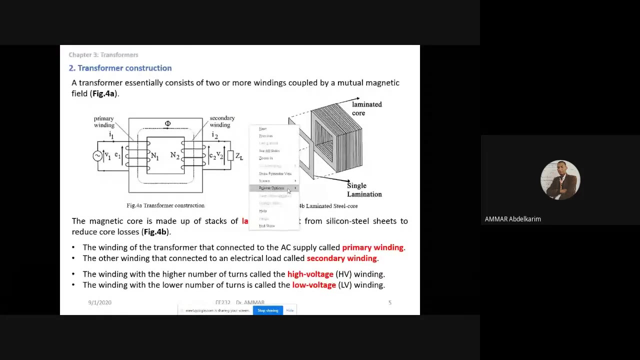 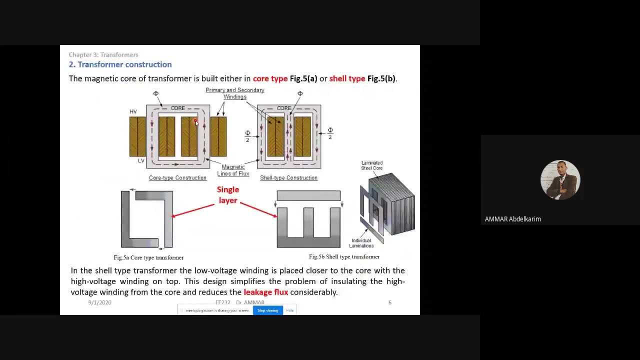 Okay, Just a moment, Just a minute, to add some of your colleagues. Okay, So we call this a core type transformer, according to the shape of this core And we see this is the primary winding and this is the secondary winding. Okay, 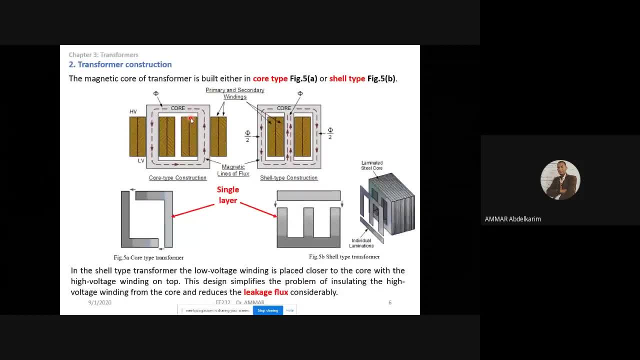 So here you are seeing a cross section of the transformer. This is the primary winding And this is the secondary winding. We call this a core type, And you see here the sheets of the core tapes, how they are made. Also we have the shell type. 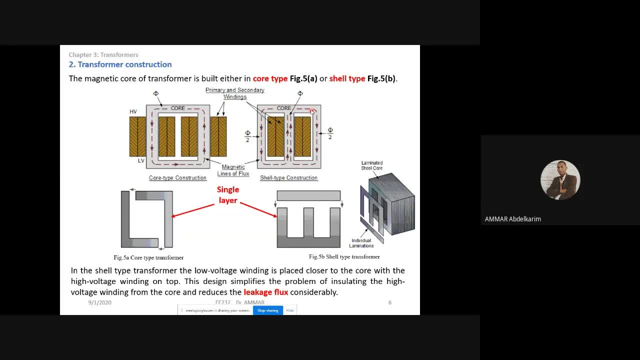 This is the shell type, which is the most used, actually the shell type. We can note here that the windings are above each other. the primary and the secondary are above each other. Okay, Okay, So they are above each other. 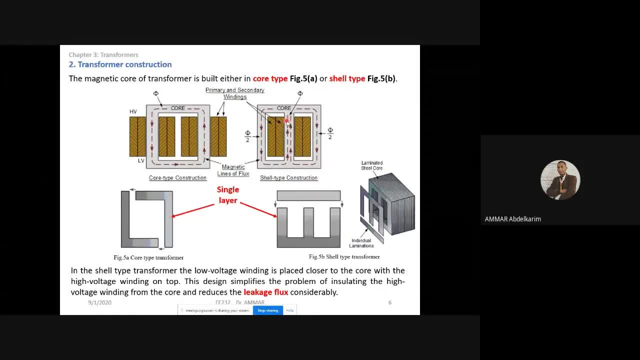 They concentrated in the middle of the core and they are above each other, So this type can reduce a lot the leakage flux. Okay, So this shell type, which is the most used, actually is used in order to reduce the leakage flux. 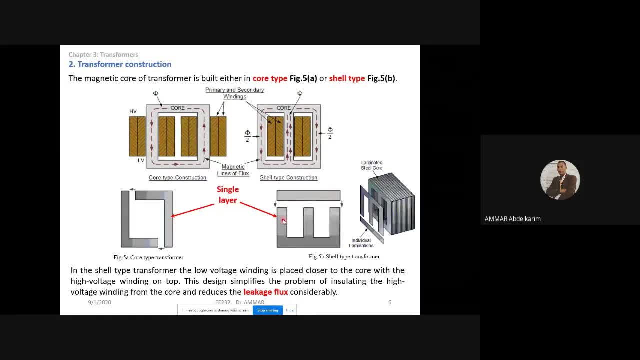 And those are the type of the lamination in the shape of E. So the lamination, The sheets of this shell type are in the shape of E And those are the lamination of this shell type. In the shell type transformer the low voltage winding is placed closer to the core. 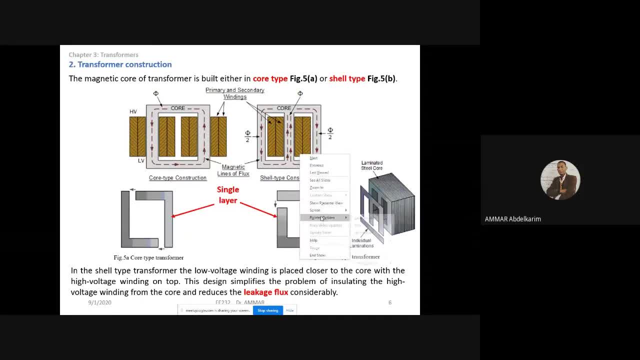 So the one here inside- Okay, Let's use the fan- The one here inside is the low voltage, The low voltage winding, And the one here inside is the low voltage winding- Okay, Let's use the fan, Okay. And the one in the top is the high voltage. 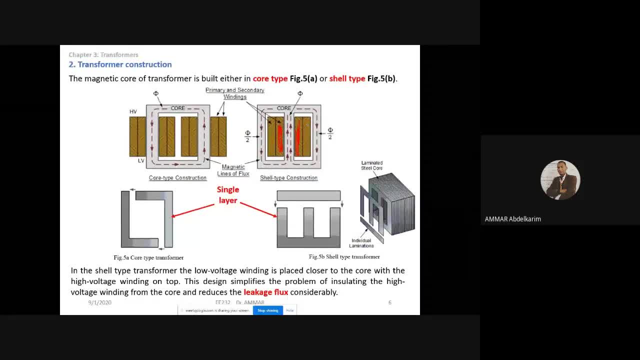 Let's change the color. The one here, this one is the high voltage current, And this, I guess, for the purpose of cooling, The cooling of the transformer, Because the low voltage winding has voltage, Of course it's high current. 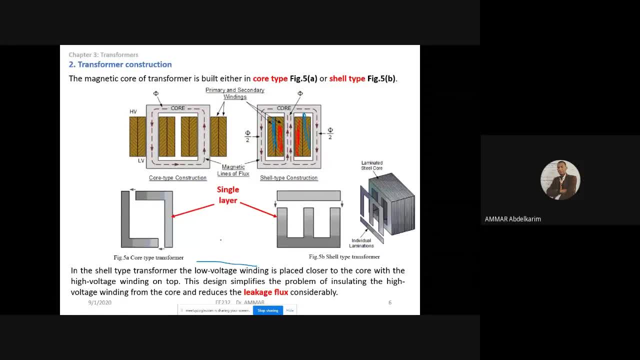 And the cross section of this winding is bigger than the high voltage winding. So this design simplifies the problem of insulating the high voltage winding from the core and reduce the leakage flux. So this shell type proposed to reduce the leakage flux And actually all the transformers. 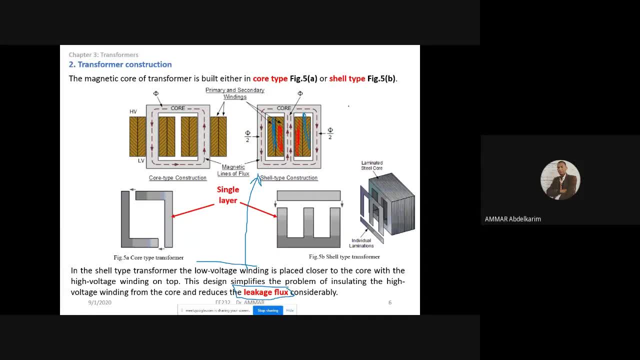 That exist are shell type transformers, But in our studies always we consider the transformer as a core type in order to simplify. But all transformers that exist today are a shell type in the shell type construction. Just a minute. Okay, Let's move on. 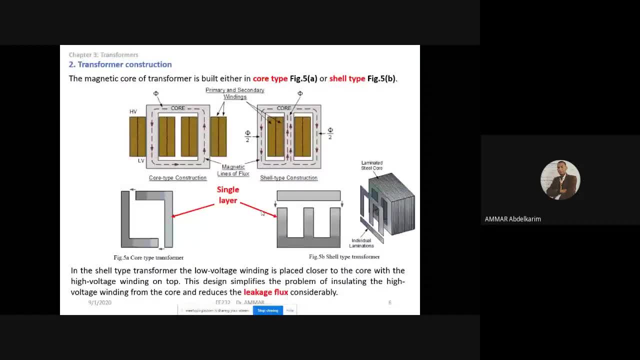 Okay, Let's move to the next slide. So, Sir, please, Yes, Can you go back to the slide. Sir, what about here in the core type, Where is the secondary and the primary? Is it the same like in? 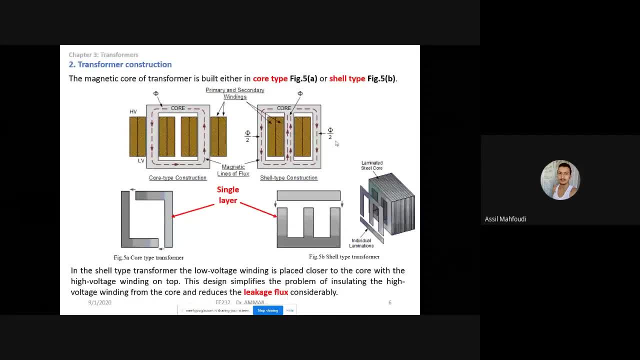 The primary is in the left and secondary in the right. No, You are not obliged. We can choose, as this one is primary and this one is secondary. It's our choice. Okay, Okay, Thank you, Thank you, Thank you. 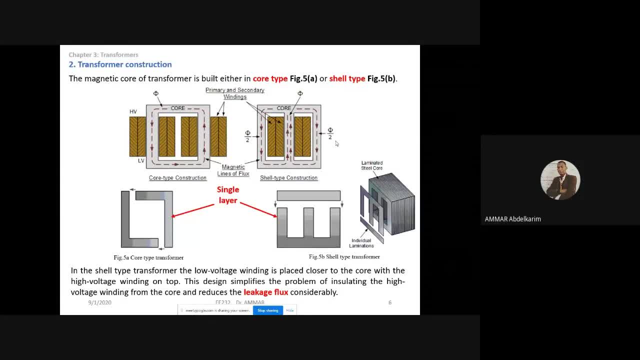 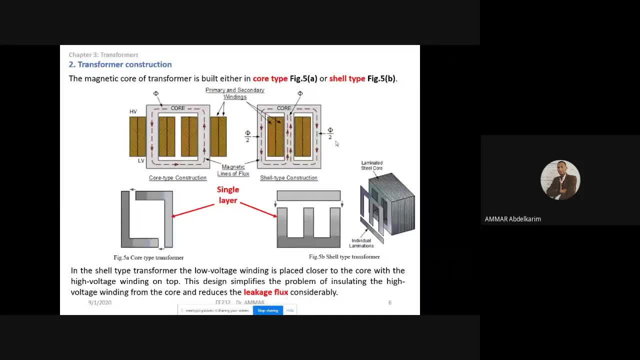 Yes, In the core type we can choose: The primary is the one connected to the source and the secondary is the one connected to the load. Okay, Okay, Thank you. Whatever, whatever we choose, which one connected to the source and which one connected? 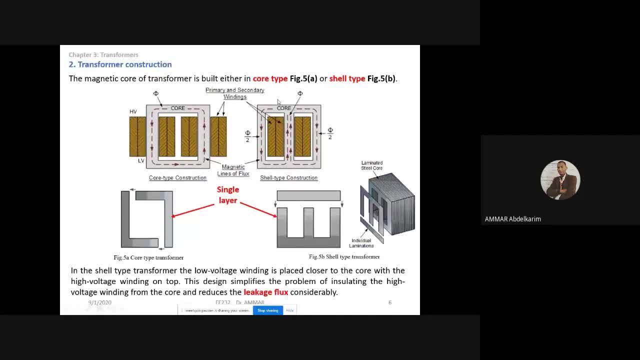 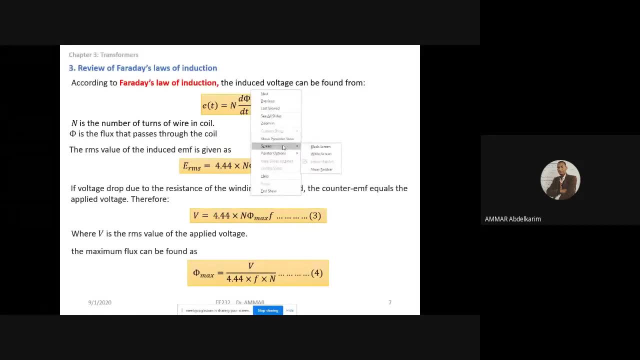 to the load. Okay, Okay, The next slide, element number three, is the review day. Yes, Yes, In view of Faraday's law of induction- we have seen this, of course, in the magnetic circuit. maybe one of the last elements in the chapter: Faraday's law of induction: the induced voltage. 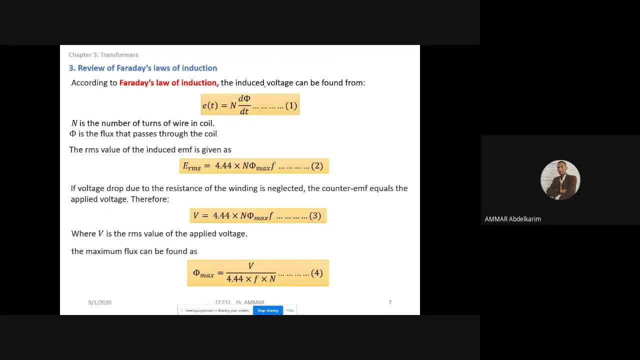 can be found. So, before we are talking about how we can produce a magnetic field or how we can have a flux- and one of the cases is when we have a time change flux. So this is why the transformer works only with AC, because transformers are based on 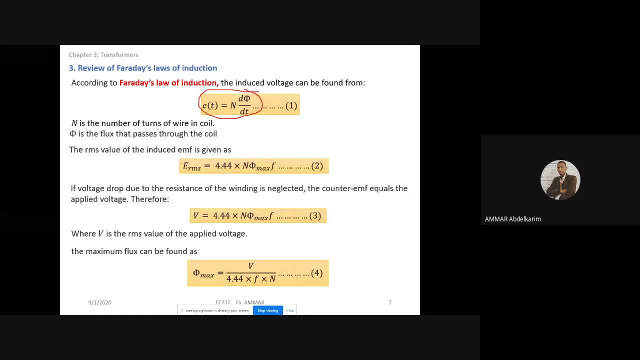 Faraday's law. So if this voltage is DC, if we give a DC voltage to the transformer, the flux will be constant And this derivative will be zero. That's why the transformers work only with AC. So according to the expression number one. so in this chapter I have added the numbering. 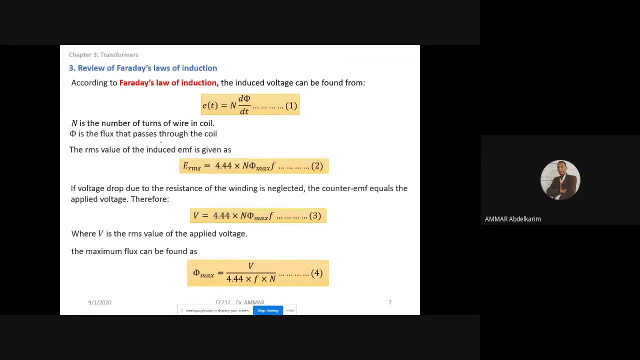 of the expressions And of course it's the number of turns. phi is the flux passes through the coil. So when we calculate the derivative of this expression- you have seen it before- we get this expression in terms of rms. voltage equals to 4.44, and 4.44 is 2 pi, 2 pi over. 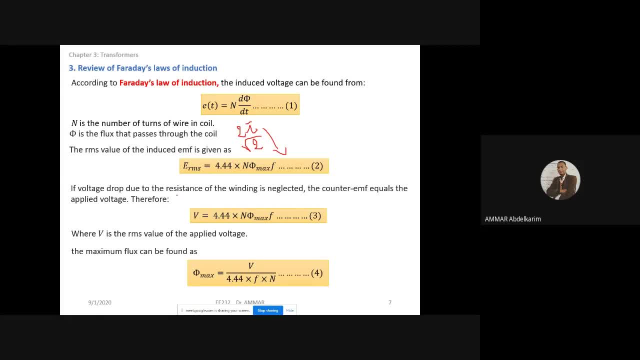 square root of 2.. This is 4.44. Times n times phi max Times, 4.44. Times f, which is the frequency And if the voltage. so this is an emf and this is a voltage. 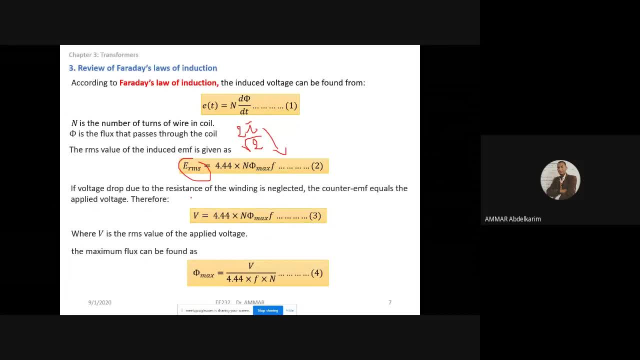 So the difference between them? we are going to see it, inshallah, the difference between real and ideal transformer. But if we consider that the voltage dropped due to the resistance, because the winding of the transformer has a resistance, Okay, So the voltage equals to the emf plus that voltage drop, which is ri. 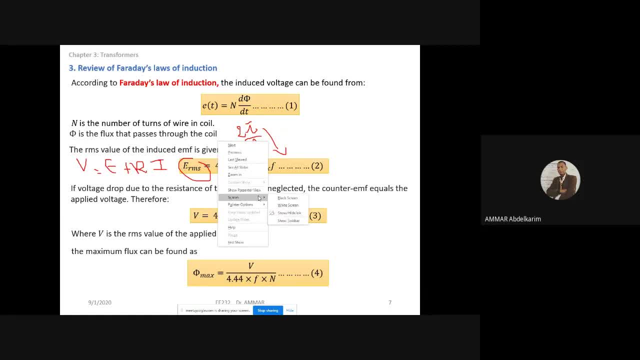 But here, if we neglect that voltage drop, the emf will be equal to the voltage. Okay, So if the voltage dropped, if the voltage dropped due to the resistance of the winding is neglected, The emf equals to the voltage drop, The emf equals to the applied voltage. 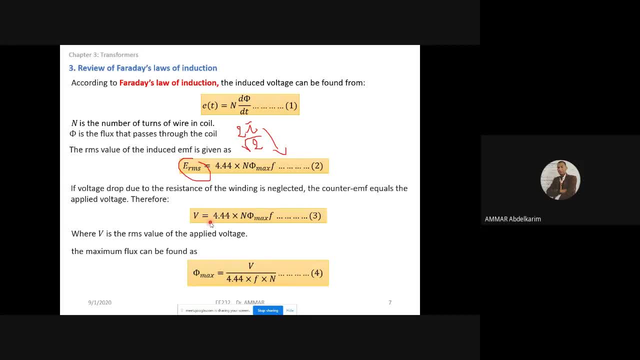 So v equals to 4.44 times n times phi, max times f And, of course, the flux equals to f over 4.44 times f times n, which is the number of turns. So why we are seeing this expression? This is the principle of operation of the transformer. 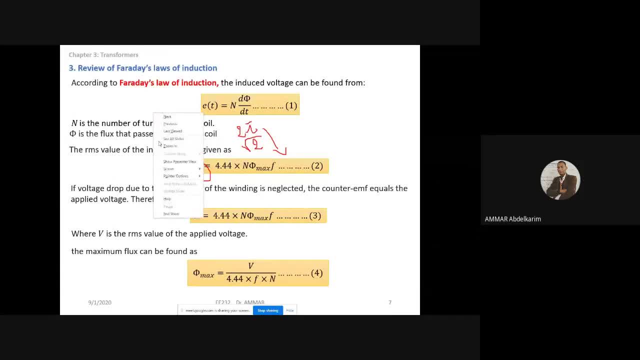 Okay, Why? Well, the flux that's produced by the flux produced by the primary winding go to the secondary winding, It will create another voltage, which is the secondary voltage, according to this expression. Okay, So this is how the flux creates. 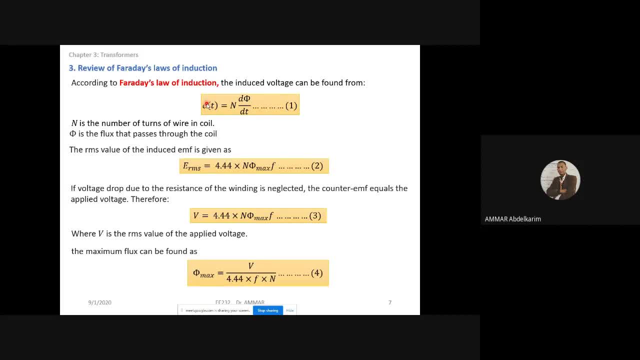 Okay, Another voltage. You asked me before how we can get an induced voltage. using induced voltage. You are using a time-changing flux And you asked me: where did get that flux? here We have flux. Why This flux came from another source. 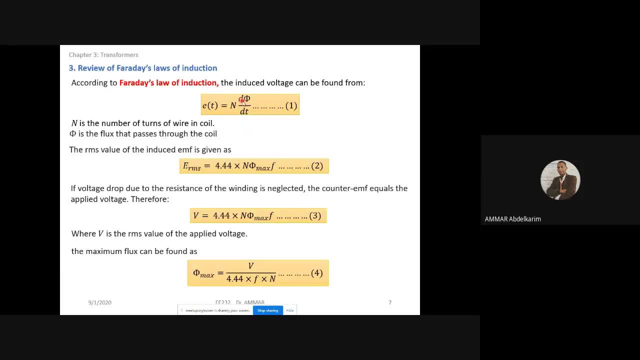 Okay, It came from the primary winding. So the flux of the primary when travel, let's say travel to the secondary, it will create another voltage according to this expression. So this is the output. voltage can be calculated according to Faraday's law. 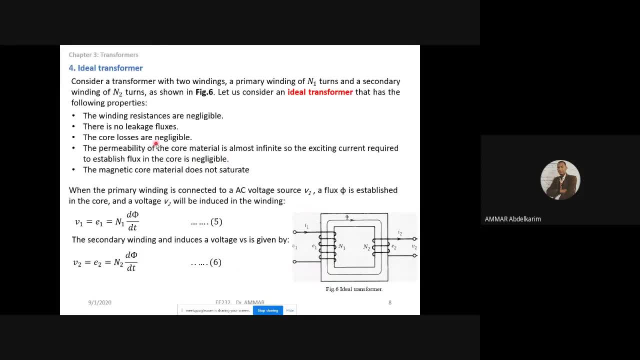 Number four: ideal transformer. So firstly, to simplify the study, Let's consider our transformer as an ideal transformer. Then we are going to see the real transformer. So of course our focus is on the real transformer, But here, to simplify study, let's start with the ideal transformer to understand such things. 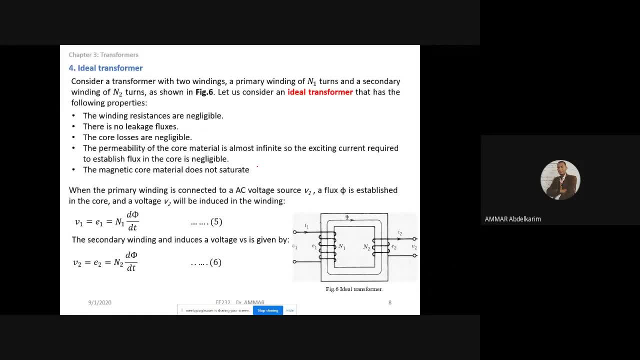 Then we pass. when we pass to the real transformer, things will not seem complicated. Okay, So let's consider the transformer with two winding: primary of N1 turn and secondary winding of N2 turns, as shown in the figure number six. here Let's consider an ideal transformer. 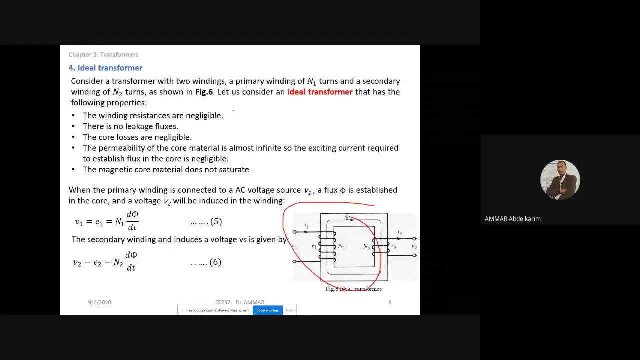 What does it mean? an ideal transformer? Firstly, the winding resistance are neglected. The resistances, the internal resistances of those winding, the primary and the secondary, are neglected, So the resistance is zero. There is no leakage flux. Okay, there is no leakage flux. 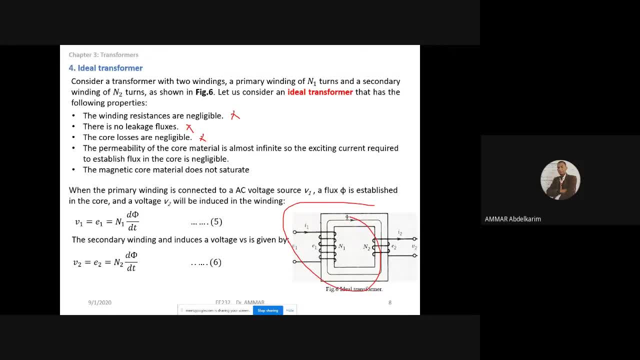 The core losses are neglected also, There is no core losses. The permeability of the core material is almost infinite. So the exciting current required to establish flux in the core is neglected. What does it mean, this passage? The permeability of the core is infinite. 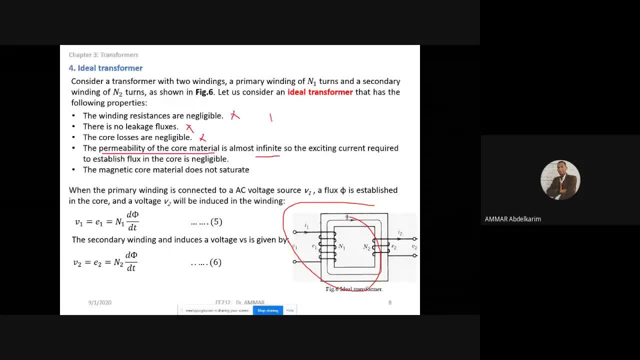 We will not have a reluctance. We know that the reluctance equals to what Equals to L over mu times A. So if this is infinite, the reluctance is equal to zero. So we don't have a reluctance in this ideal transformer, because the permeability of the 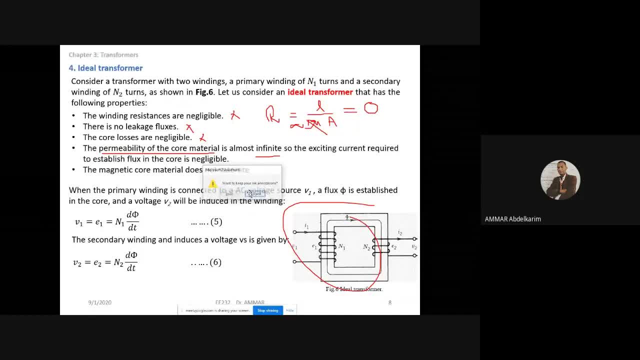 core has an infinity And if infinite value, Okay. And also the magnetic core material don't saturate. So you have seen before the magnetization curve, So the saturation point here it's not considered, So this material does not saturate. 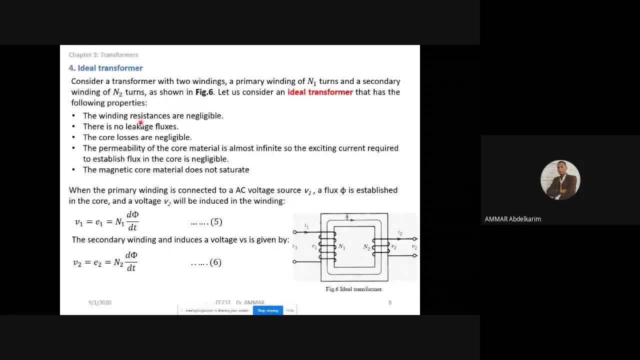 And this we call this assumptions for the, yet They are not real in reality. We don't have this. Maybe in such cases, if we use specific materials, But in general we don't have those. There is no material that does not saturate, or material without resistance or whatever. 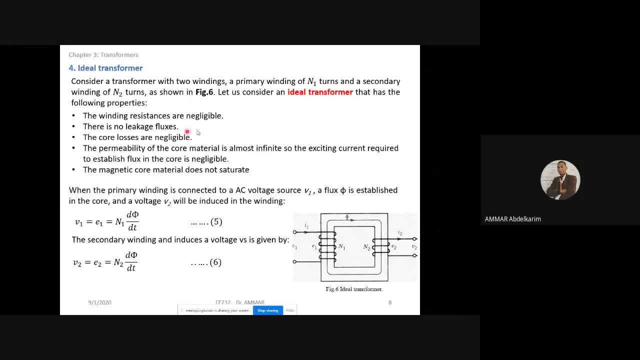 it is small, Okay, So those are assumptions for the yet. Okay, In order to simplify our studies Before, Before we get into the real transformer. So those are assumptions, So you should save them in your mind When we have an ideal transformer. 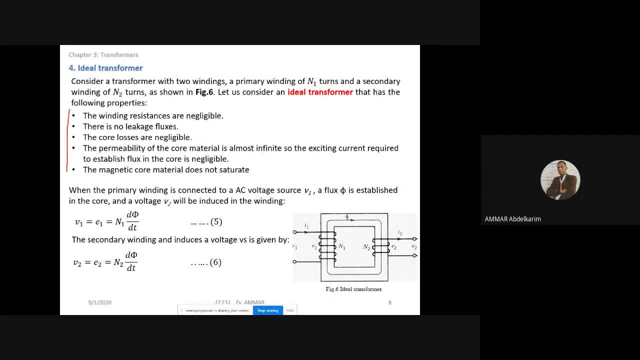 Okay, So when the primary winding is connected to the AC voltage source V1.. When we have a voltage here, a voltage source here in the primary A flux is established. So the voltage of the source will establish or create a flux in the core. 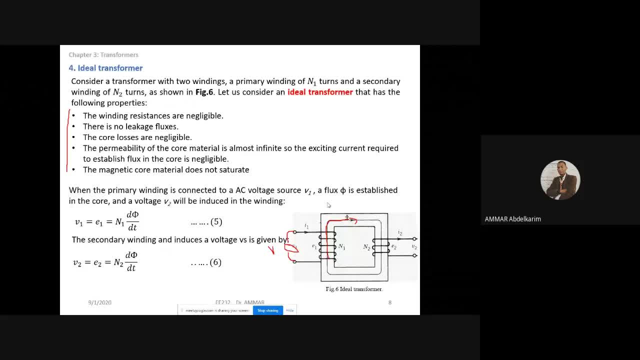 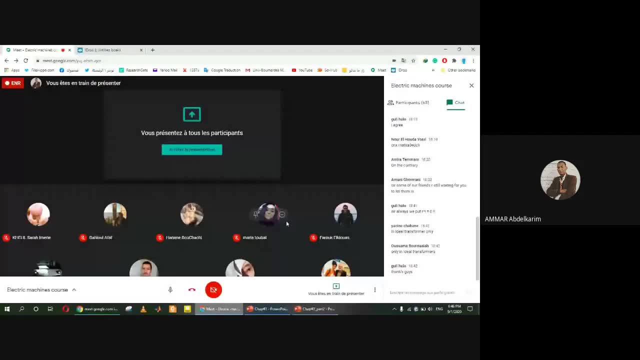 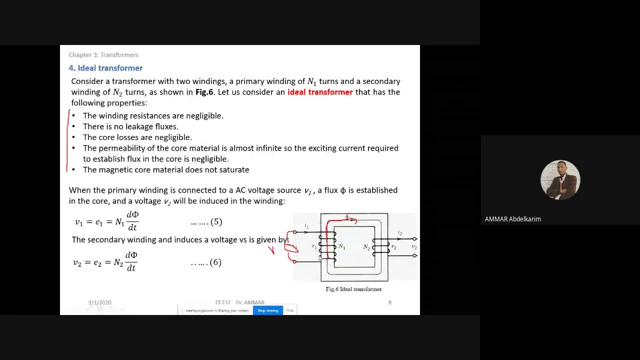 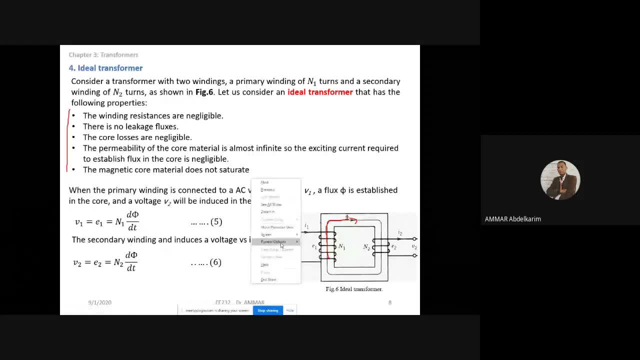 This is the principle of operation of the transformer, So the primary and the secondary are not connected physically. There is no wire, for example, between the primary and the secondary. That's why we use transformers for isolation. They are not connected physically. 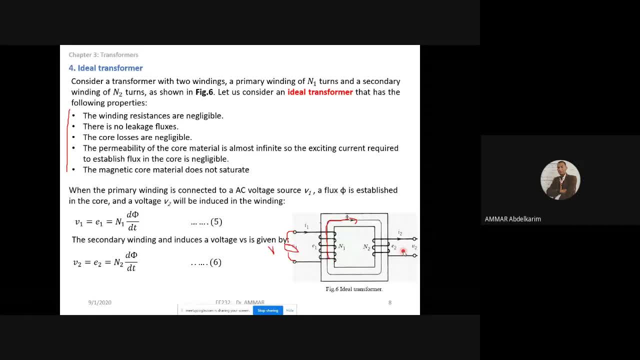 There is no wire, for example, between the primary and the secondary isolation. they are isolated only the flux which transfer from the primary to the secondary, the voltage of the source, creates flux. here, of course, here, in the ideal transformer, we are neglected the leakage flux. so these flux, the linkage, 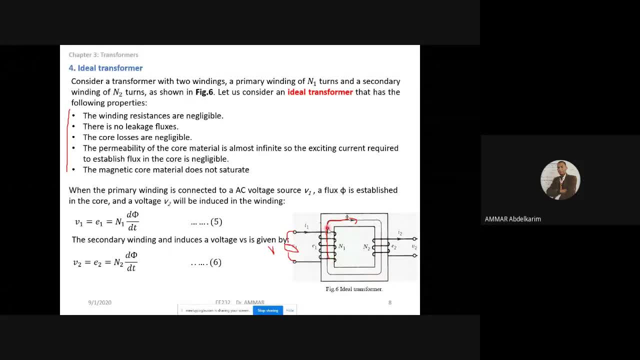 flux that's created in the core, when it travels to the secondary it will induce another voltage, which called a secondary voltage. so this is the voltage expression of the primary voltage, number five. a flux Phi is established in the core and the voltage V2 will be induced in the winding, the secondary winding. 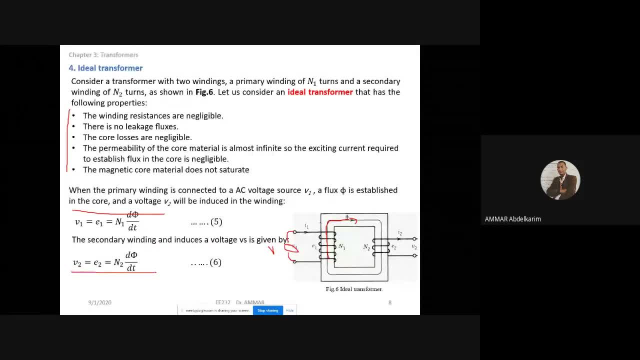 induced voltage is given by this expression: yes, okay, so this is the principle of operation of the transformer. I will repeat: the voltage of the source will create a flux in the core. then this flux, when it transferred to the secondary, it will create another voltage. so here the 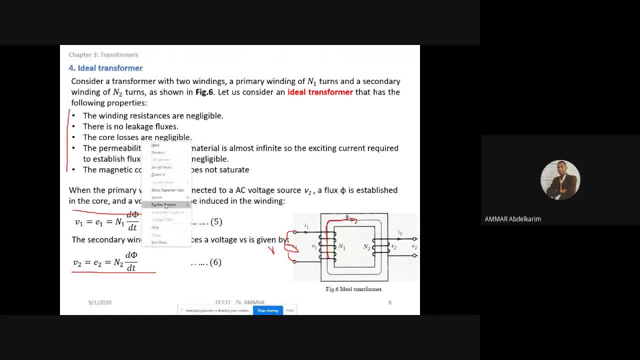 difference because here we have the same flux. of course it's the same flux that transferred it from the primary to the secondary. but the difference of the amount of the voltage of the primary and the secondary depends on the number of terms. so V1 equals to e1, equals to n1. d5 over dT, V2 equals to e2 equals to n2. 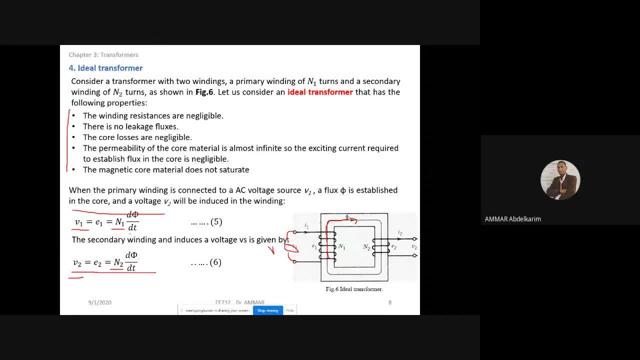 times dV over dT. the same flux, but the number of terms is different. so the number of terms of travelled is equal to the output we used before, and vs the and into Pr1 times dT. Nicholas Gustafsson, Stephanie Rogoff, Story tiethe Мы sittenicy кур openlyMAN Nedim. 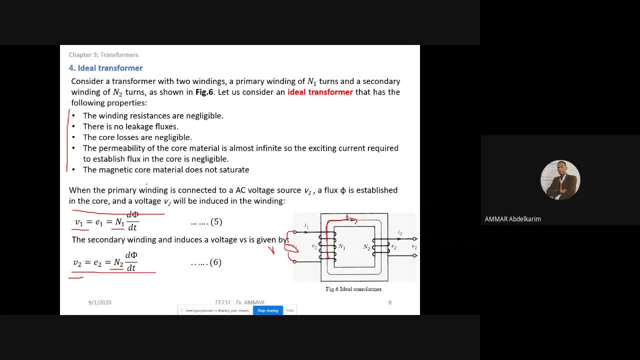 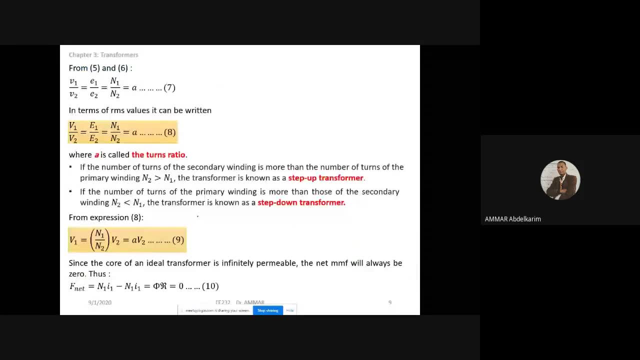 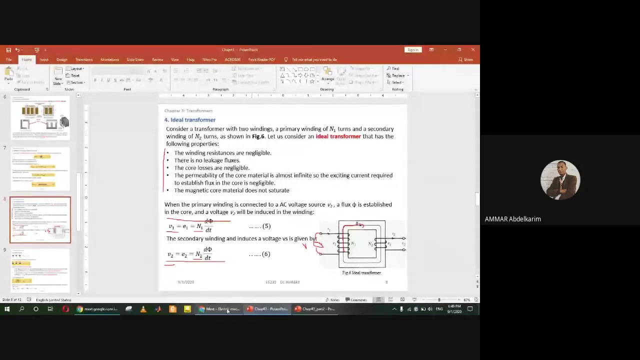 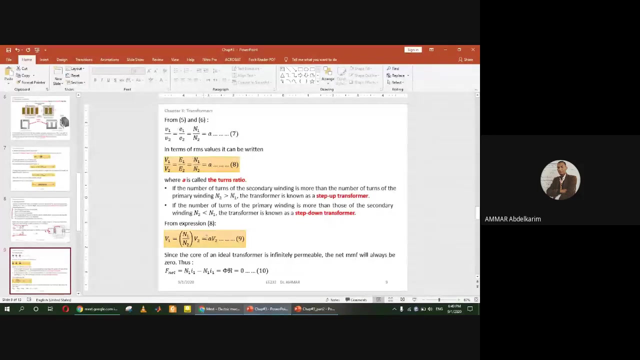 the voltage is different. okay, let's move to the next slide. so, from five, from five and six, we can write in this expression: so if we divide those expression part by part, okay, so let's go to the table, okay, okay. so here, from five and six, we have v1. 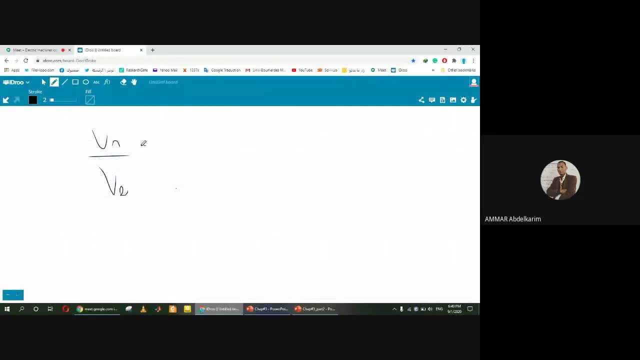 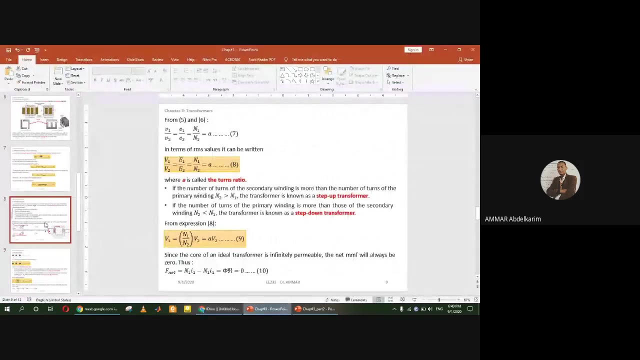 over v2 equals to e1 over e2, and this equals to e2, and this equals to e1 over e2 and this equals to n1 over n2. from from those expressions five and six, v1 over v2 equals to e1 over e2, equals to n1 over n2. 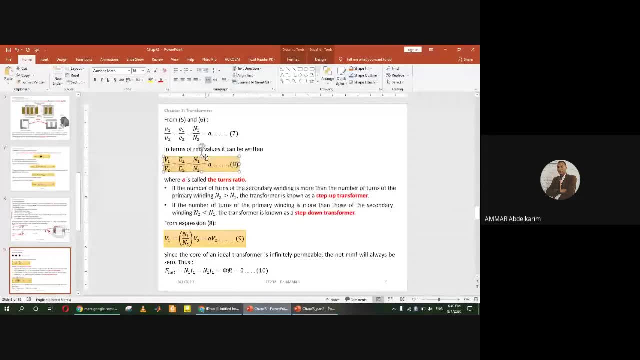 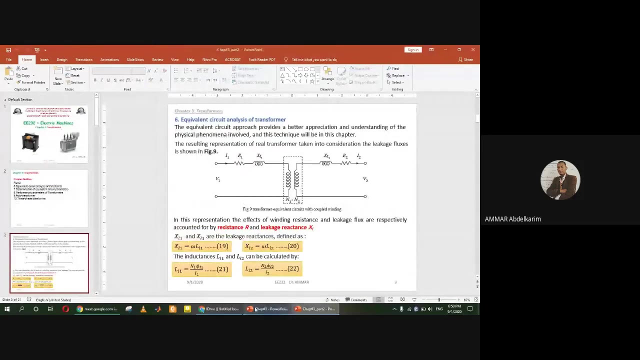 so here in number eight are written in term of rms. so here the small letters are instantaneous values and the capital letter are rms. so here the small letters are instantaneous values and the capital letter are rms. okay, no problem. so let's work with rms values. so this, this report, we call it the terms ratio a. 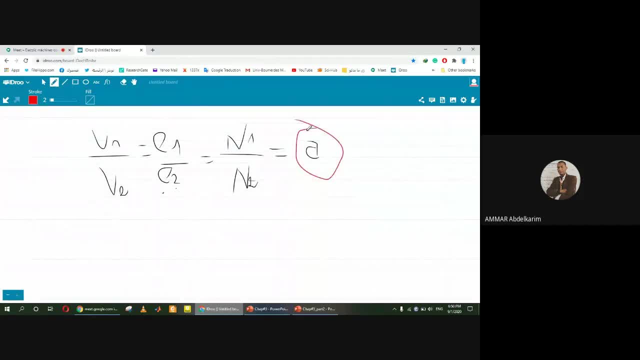 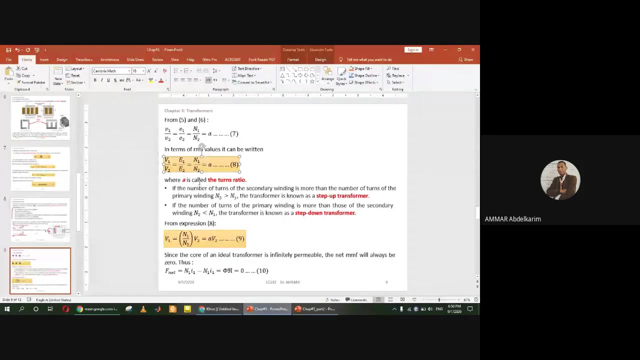 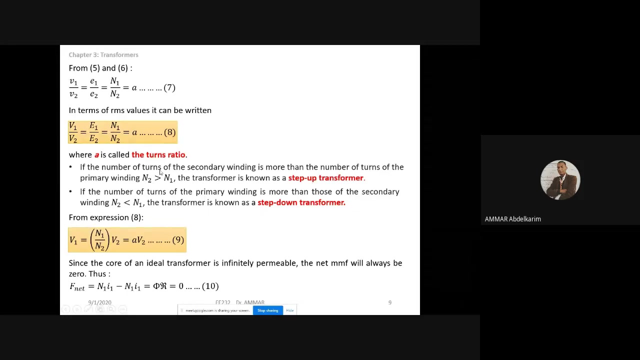 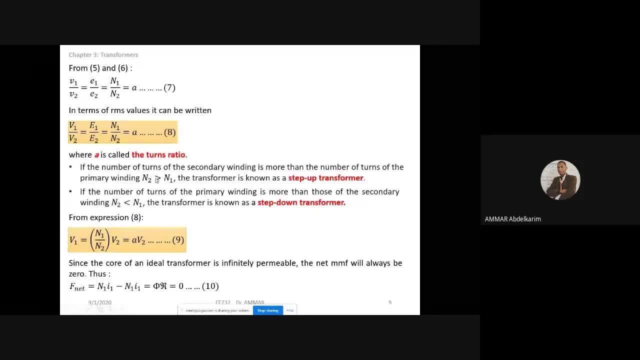 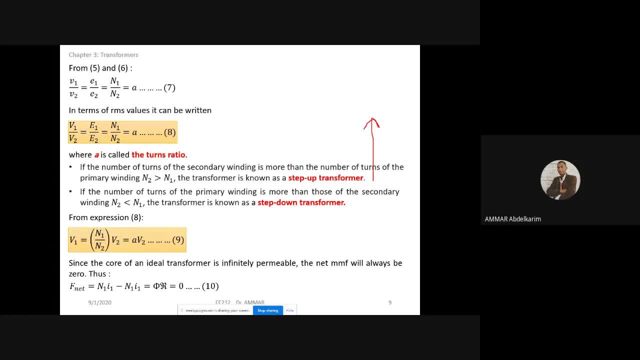 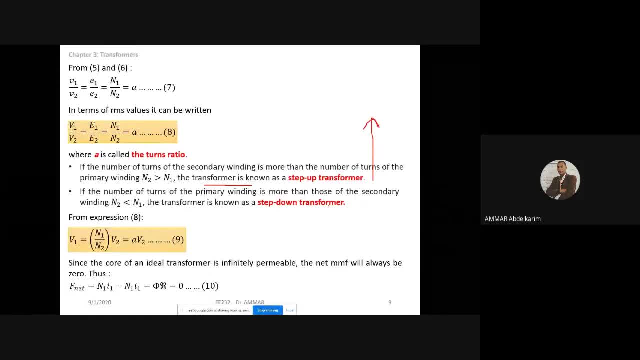 So N2 less than N1, this transformer called step-down. Okay, Step-down, which decrease the level of the voltage. So, using the expression shown in 8, and in order to prove this, Y, when N2 greater than N1, we call it step-up, and when N2 less than N1, we call it step-down. 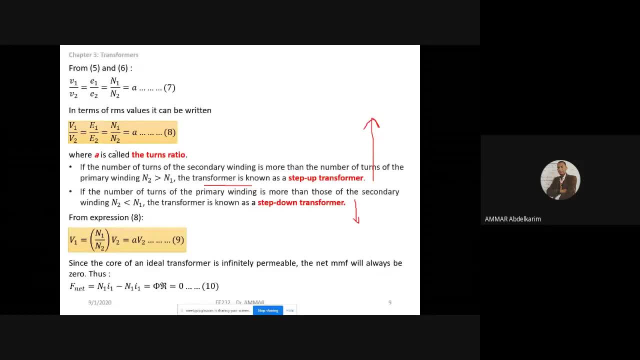 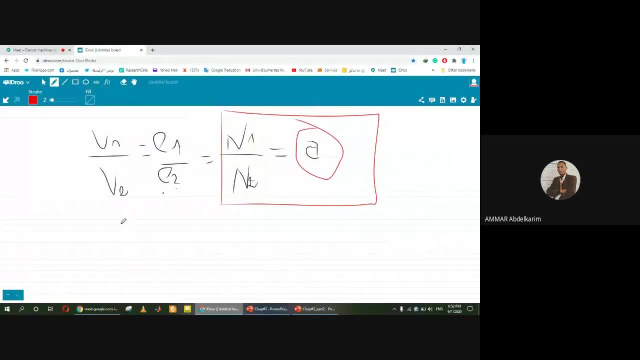 So, using this expression, let's go to the table. Using this expression, of course, we have V1 over V2, equals to N1 over N2, and this equals to A. And this means what? So let's take this equality. 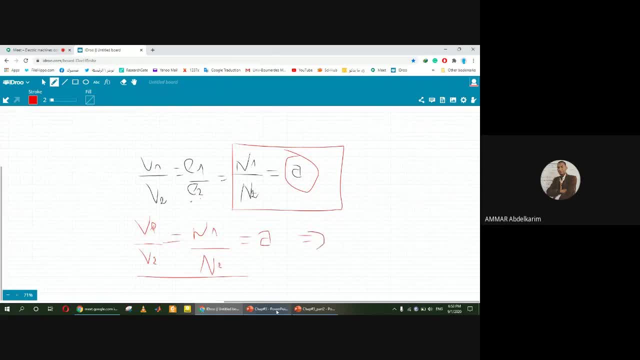 This means that V1 equals, equals to what Equals to V2 times N1 over N2.. Okay, Okay, And equals to what V1 equals to V2 times A. So if, if N1 is bigger than N2,. 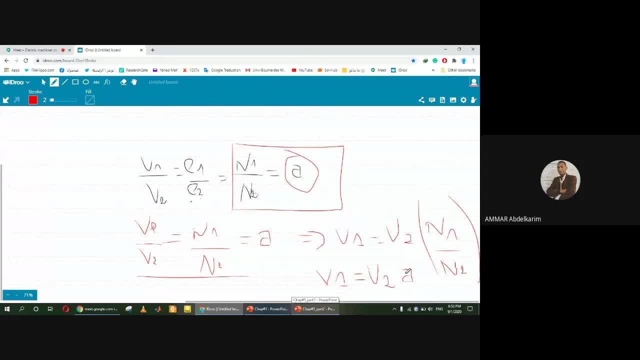 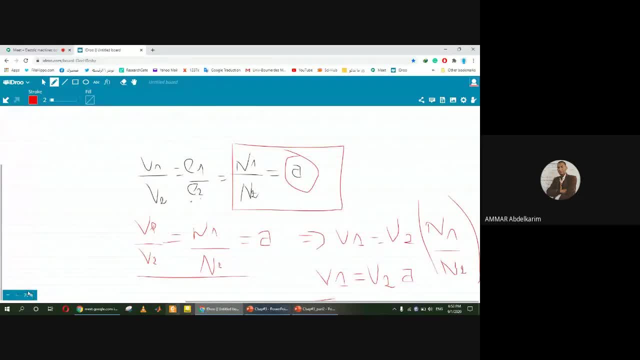 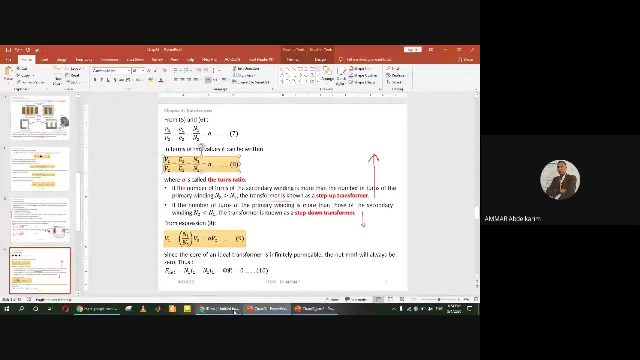 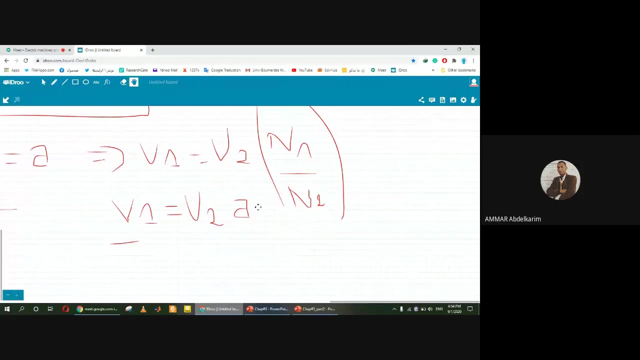 Okay, Just please focus on this. You may see it complicated, but it's not Okay. So, if N1 is bigger than N2, if N1 is bigger than N2, than N2, which means that this transformer is a step-down transformer. 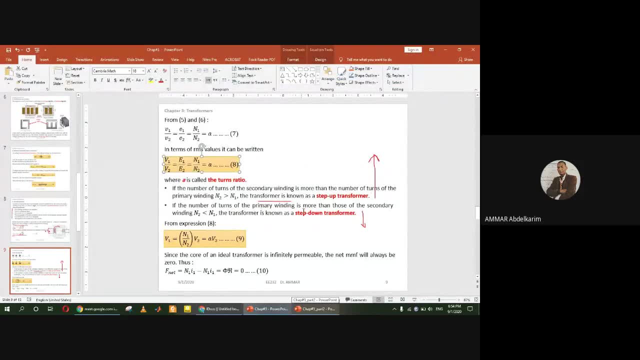 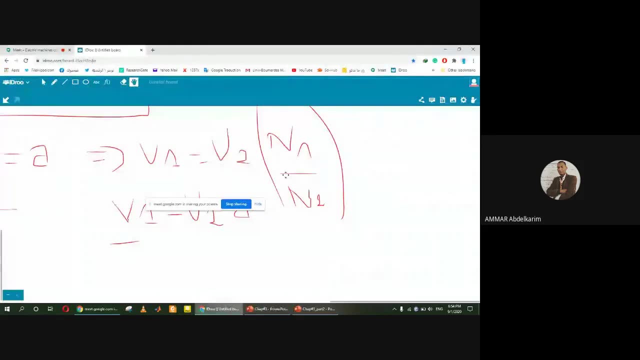 As we have seen here, if the number of turns primary is more sorry. so if the N1 bigger than N2, A A more than 1, which means that V1, V1 is more than V2, because here V2,. 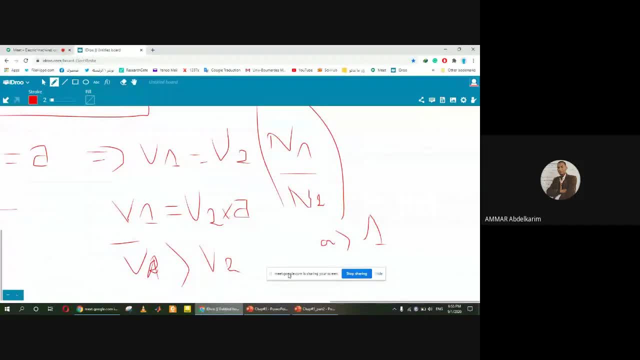 the amount more than 1,. okay, Have you get it or not? Or should I repeat it? Because this is the main objective why we study the ideal transformer. to explain the meaning of the turns ratio. okay, So we said that V1 over V2 equals to N1 over N2.. 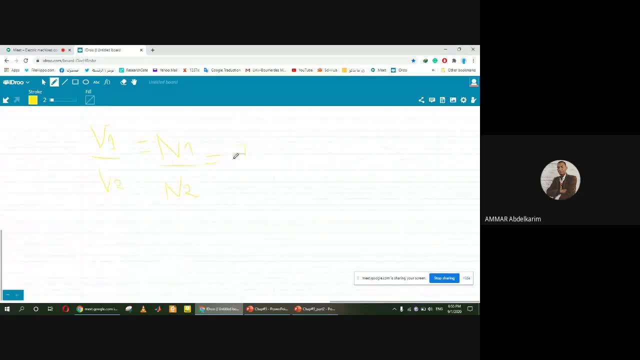 Equals to N2.. Okay, Okay, let's change the color. Equals to A, And we said that if N1 more than N2, the transformer is step-up. Those are the conditions. If N1 less than N2, this transformer step-down. 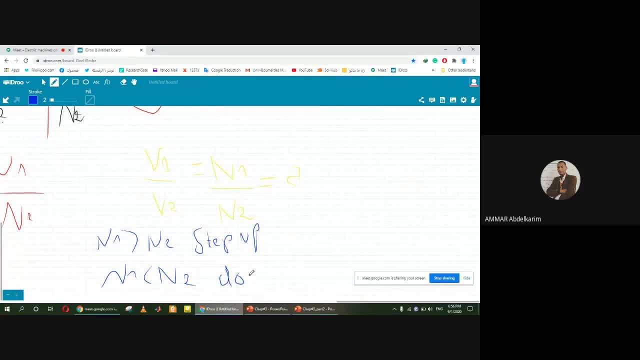 So N1.. Okay, So if N1 less than N2, this transformer step-down. So if N1 less than N2, this transformer step-down. So if N1 less than N2, this transformer step-down. 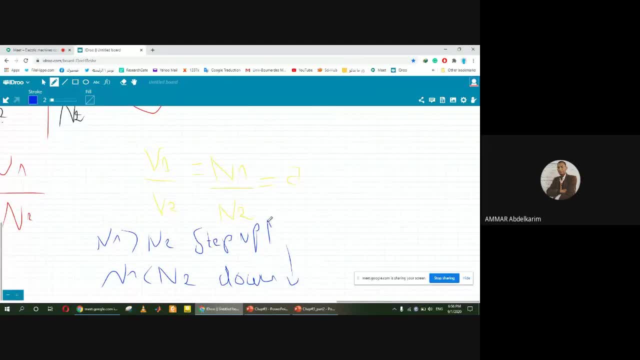 So let's write it. Let's write it like this: Step-down And step-up. Okay, So if N1 is more than N2, this equals to what It can be written like this: Equals to V1, equals to A times V2.. 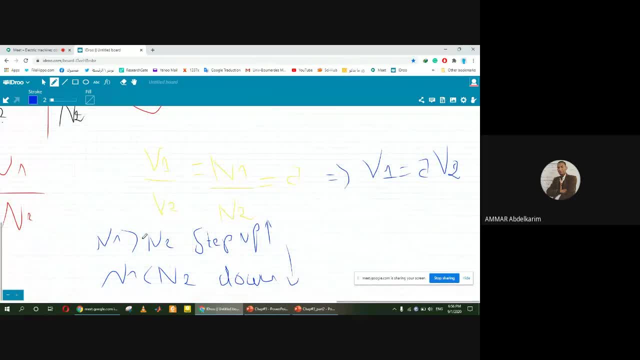 So, if N1 more than N2, this ratio, This ratio A, Okay, This ratio A is more than 1, and, of course, according to this equality, V1 is greater than V2, and this transformer, so V2 is less than V1, so this transformer is a step-down transformer. 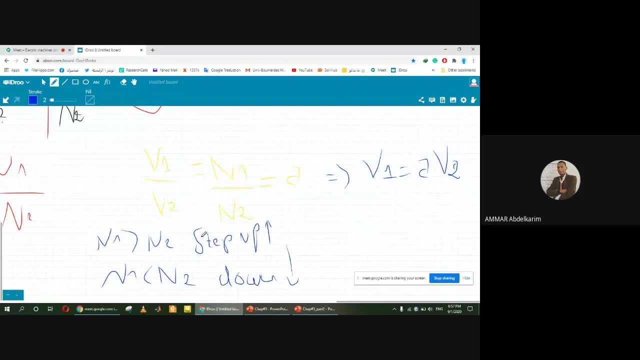 But if N1 is less than N2, this becomes less than 1.. It's between 0 and 1.. So here V1 equals to A times V2, and A is less than 1, which means that V2 is greater. 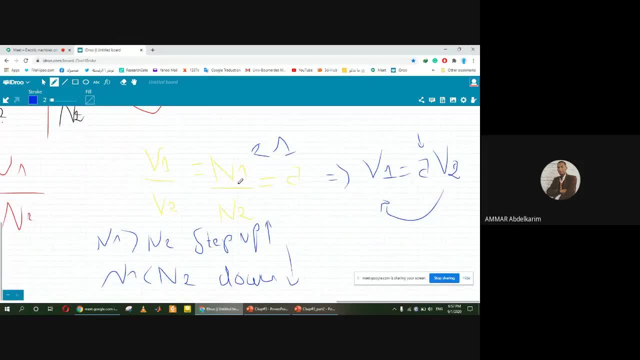 than V1.. And this transformer is a step-up transformer, a step-down transformer. Okay, Okay, Okay, Okay, Okay, Okay. Have you get it? or should I repeat it before moving to the next element? Yes, Yes, Can you repeat it please, sir? 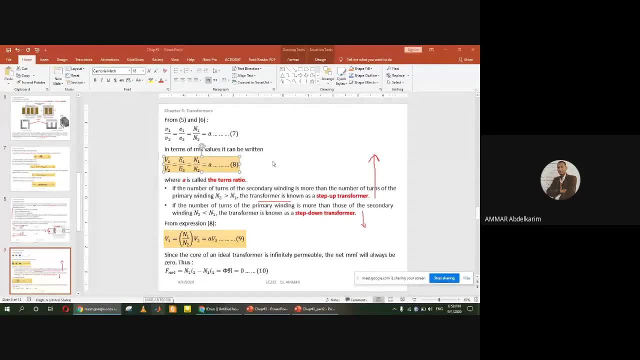 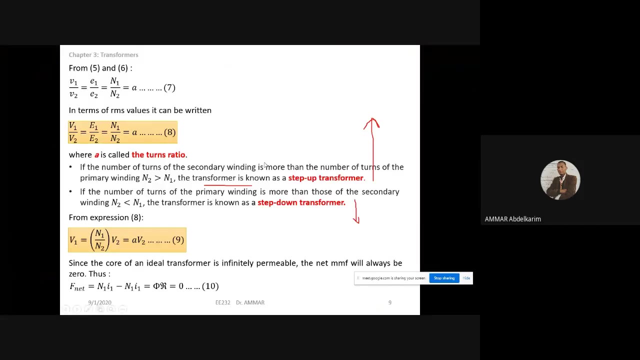 I had a problem. I know that you have such ambiguity concern. I know This is the objective of studying the ideal transformer, because if it was real we will have voltage drops, So this will not be exact. okay, that N1 over N2 equals exactly to V1 over V2, because we have voltage drops. 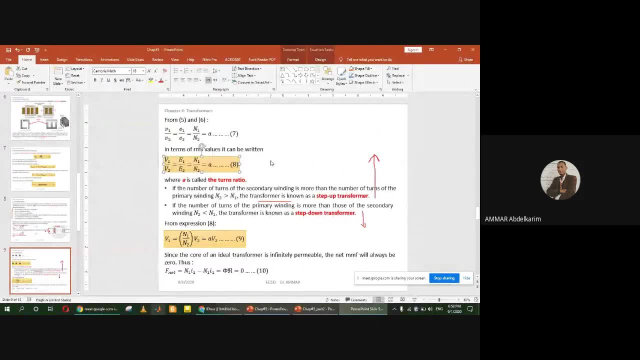 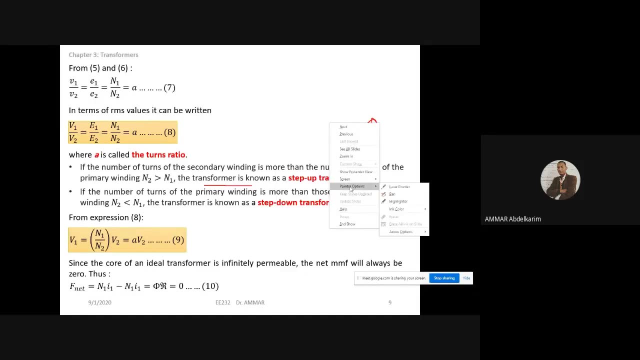 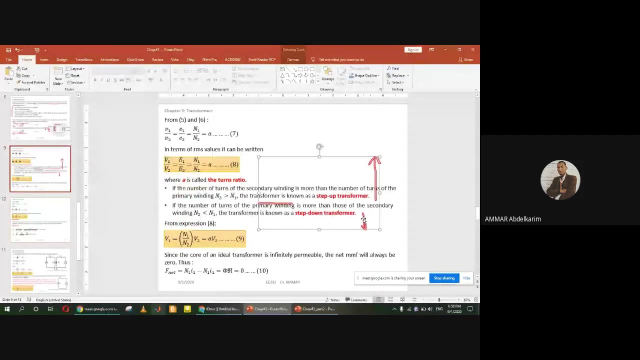 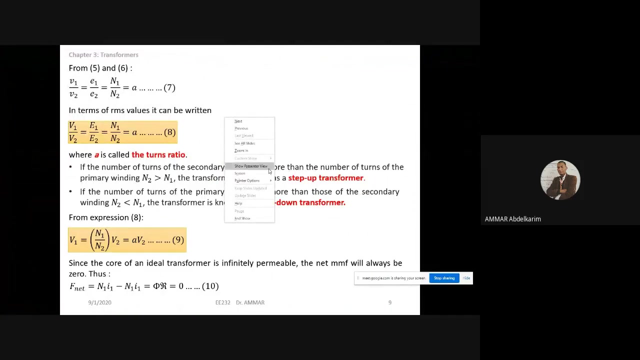 But in the ideal transformer, since we don't have voltage drops, we study the reason why we cannot raise this. okay, So let's use the pen here. Okay. so, starting from this, V1 equals V1 over V2, equals to E1 over E2, equals to N1 over N2, and we call this a turn ratio A. 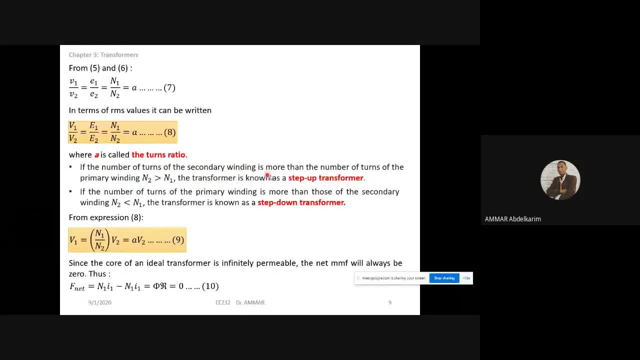 So if the number of turn secondary winding is more than the number of turn of primary winding. if So, the first case: if N2 is more than N1,, N2 more than N1, which means A, A less than 1.. 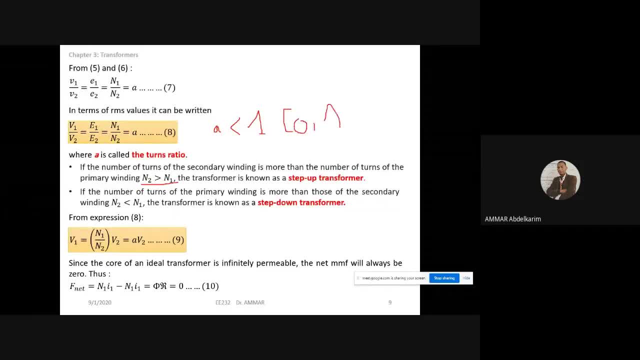 A between 0 and 1.. Okay, this is the first case. The transformer is a step up. Why it's step up? Let's take this Okay from this. we can get this Easily. we can get this. So here. V1 equals to what? 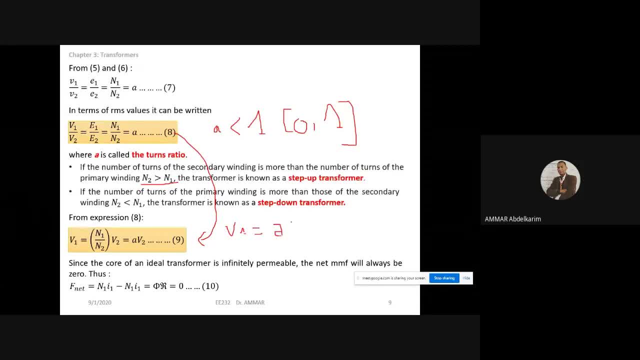 Equals to A, V2.. A is less than 1. So, according to this, V2 is greater than V1.. V2 is greater than V1 because V2 is The coefficient is less than 1. So it equals to V1, okay. 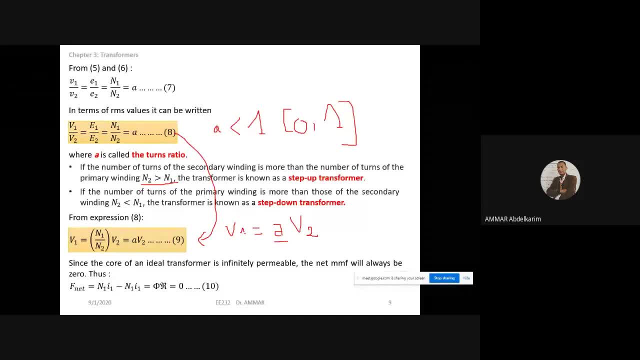 Here we reduce V2.. We can write it like this: V1 over A Equals to V2.. And you know, when we divide by something less than 1, the result will be bigger, More right. Okay, Yes or no? 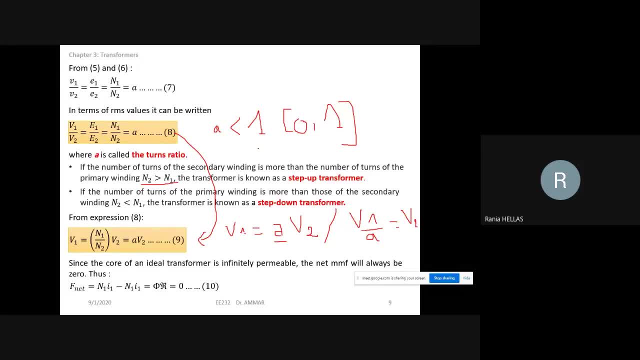 Yes, Yes, Yes. Okay, So this is the first case- If N2 more than N1. Which means that A, the turns ratio is between 0 and 1, V1 equals to A V2, or we can say that: 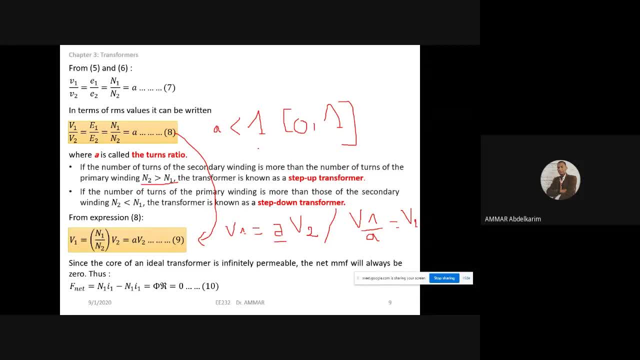 V1 over A equals to V2.. So here the voltage, the output voltage. of course, V1 is the input, which is the primary, and V2 is the output, which is the secondary. Okay, V1 over A. which A here is less than 1, it's between 0 and 1, V1 over A equals to V2.. 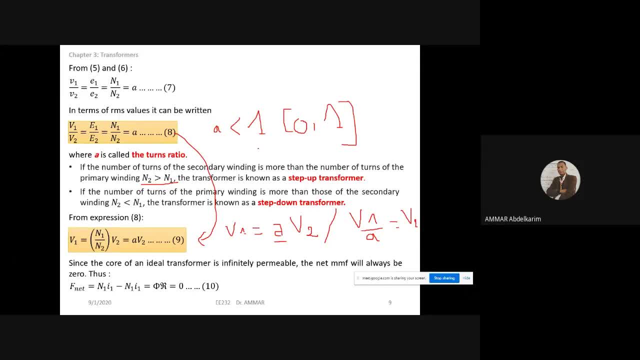 So the output is more or greater than the input. The second case, when N2 less than N1. So if N2 less than N1. So A is more than 1. 1.234, we don't know. Okay. 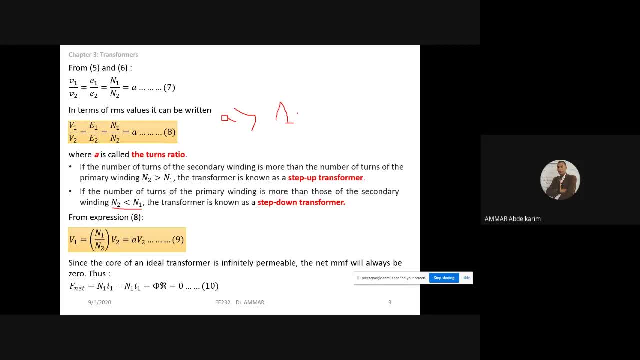 Maybe you can assume it. You can replace A by any value and you will get it Okay. So if A more than 1, V1 equals to what? V1 over A? it's the same, like this equals to V2.. 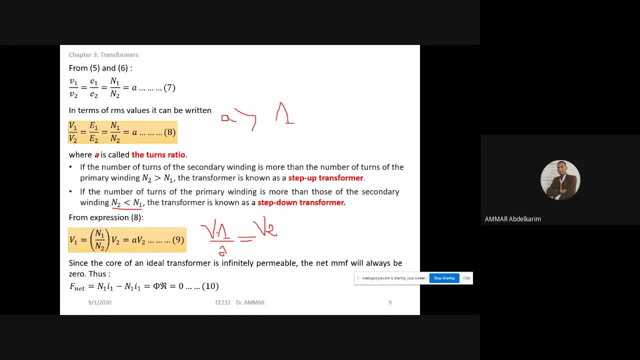 So if we divide V1 over a value more than 1, the result will be less than V1.. Okay, I think we should have an example to understand it, Okay. Okay, Let's take the simplest example we can, Okay. 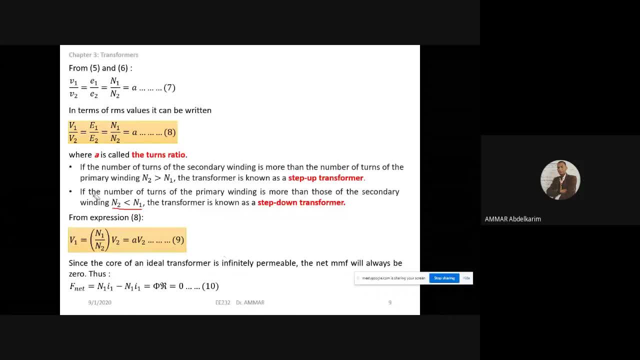 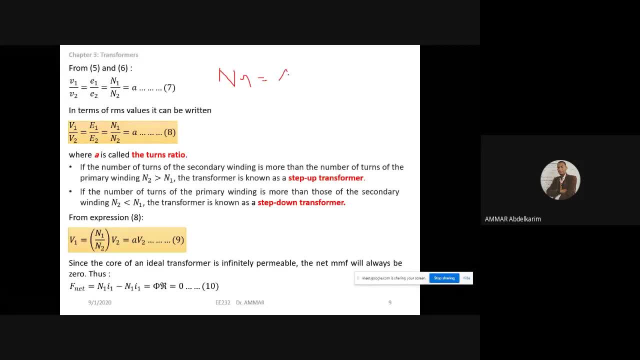 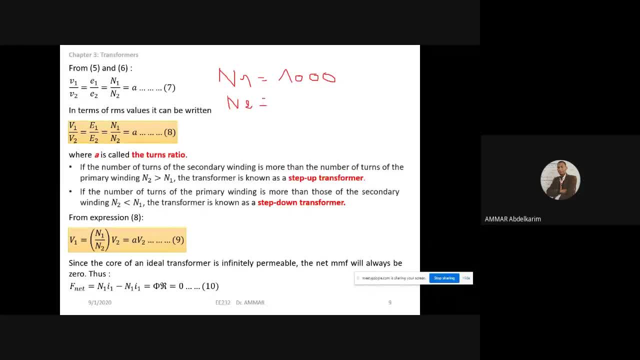 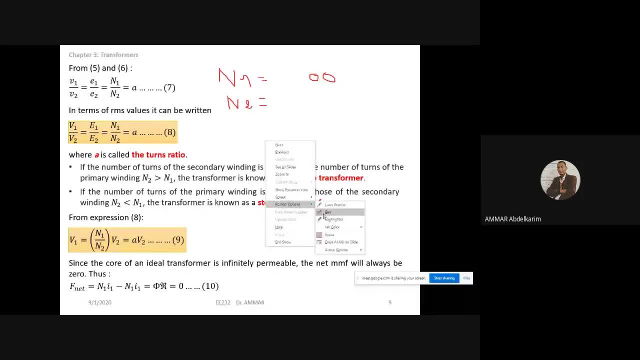 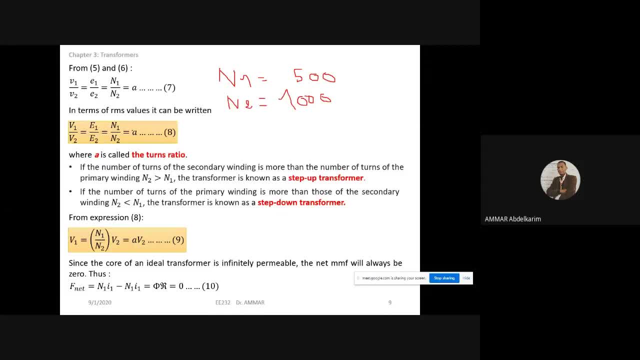 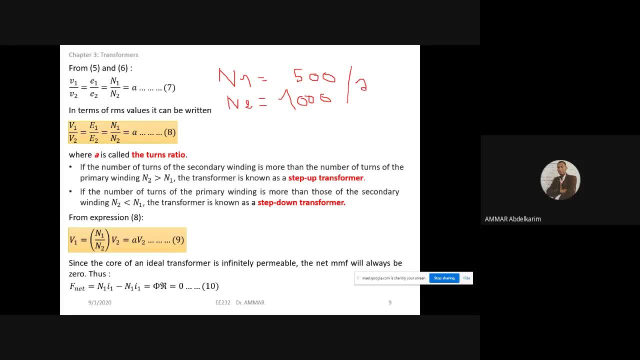 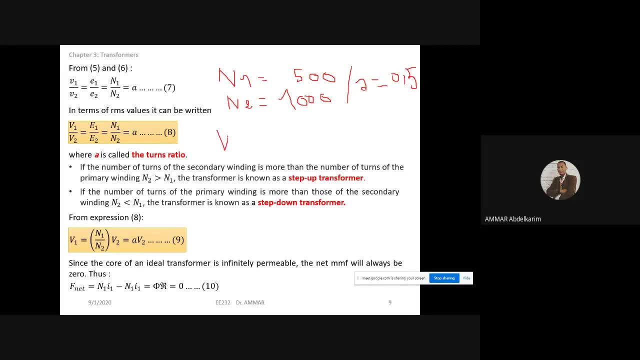 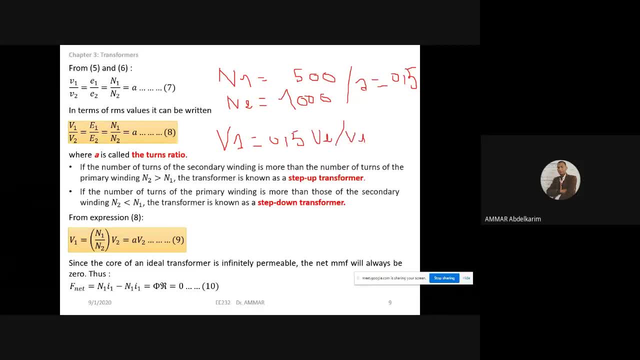 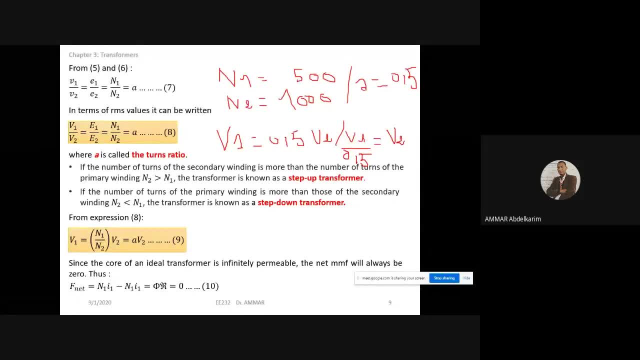 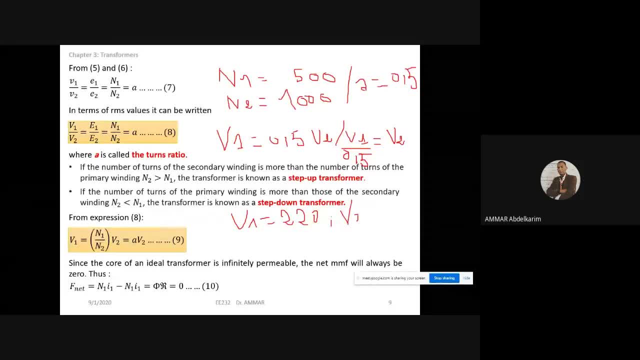 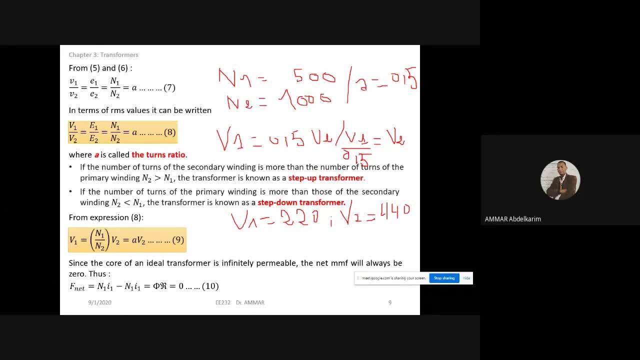 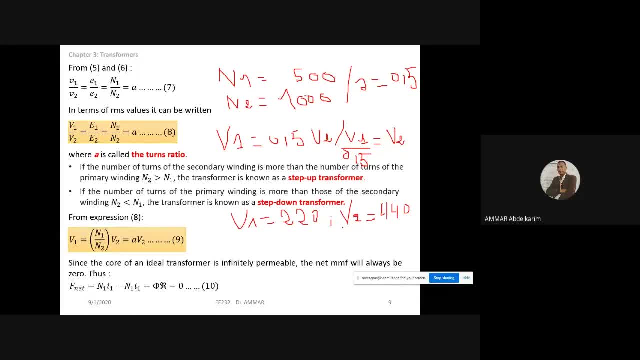 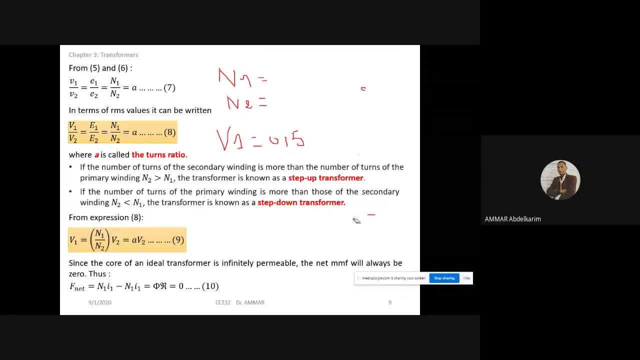 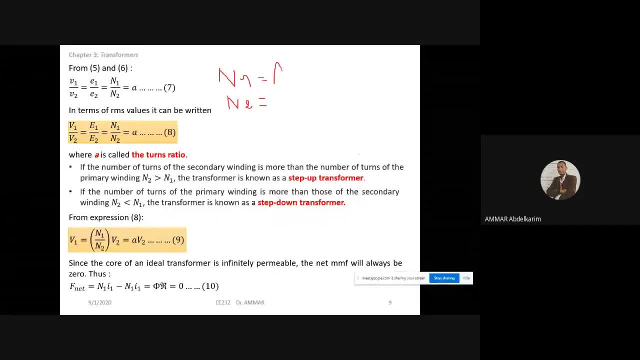 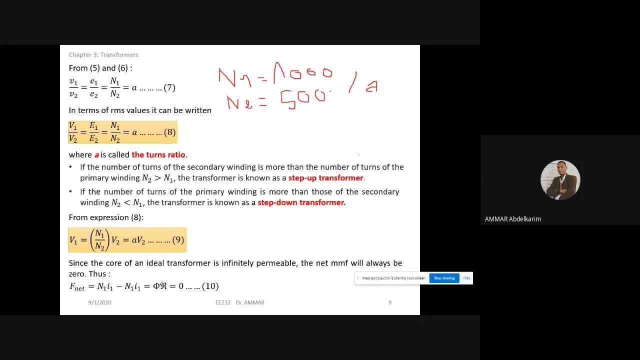 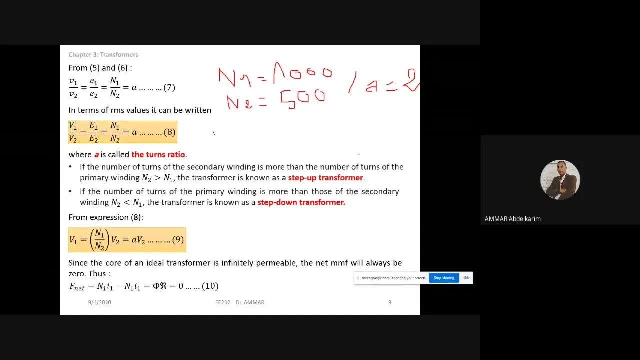 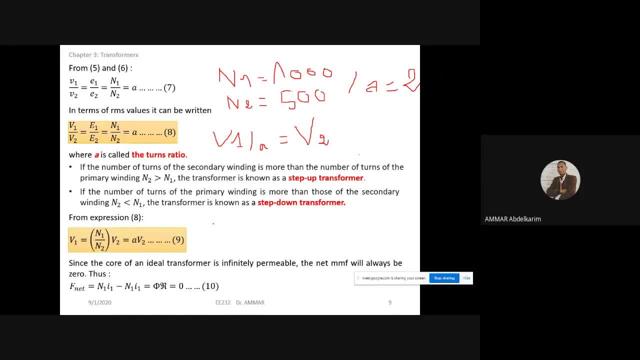 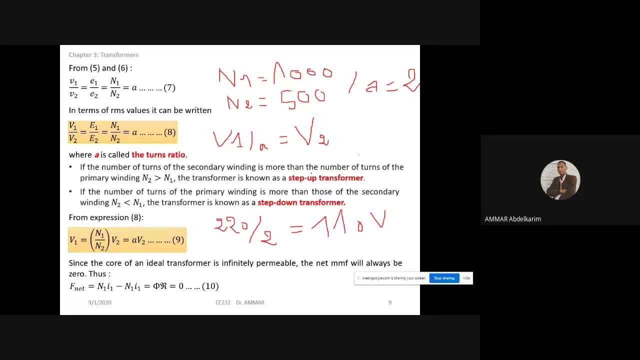 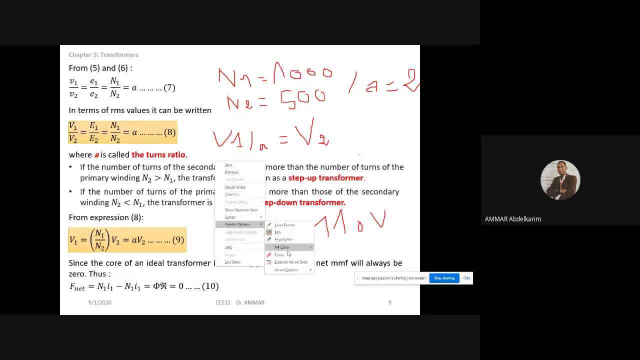 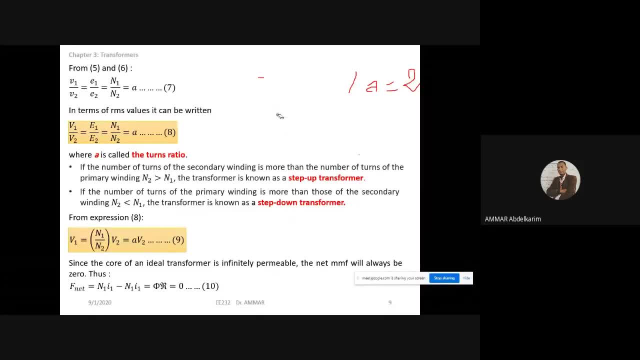 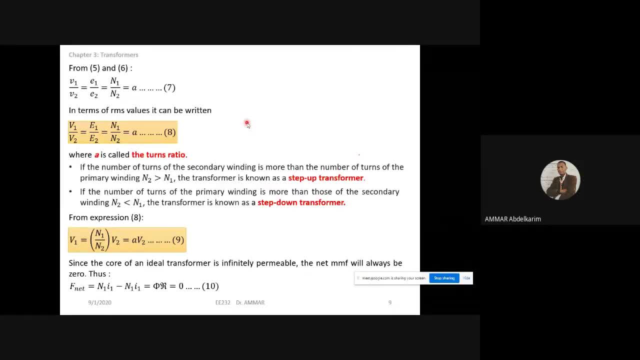 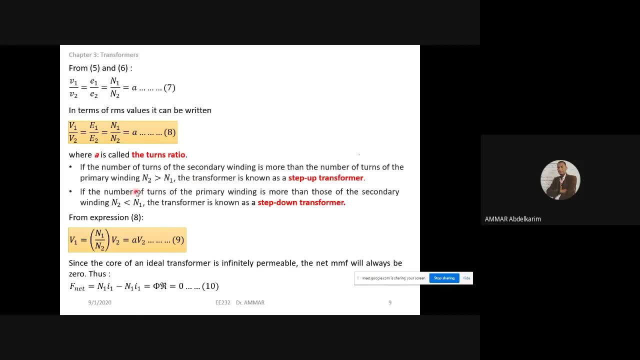 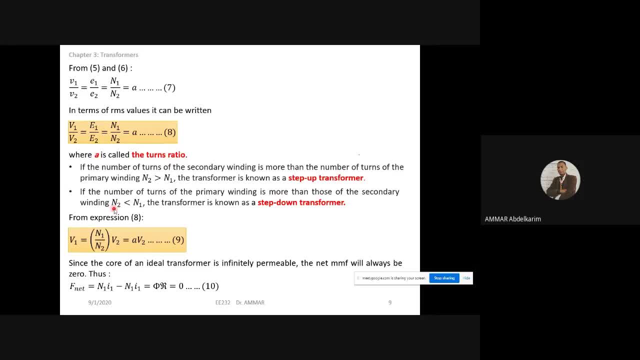 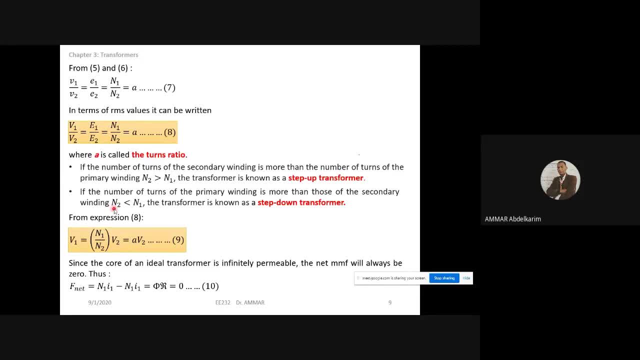 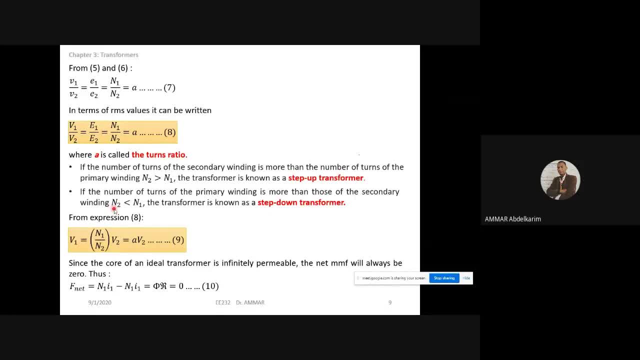 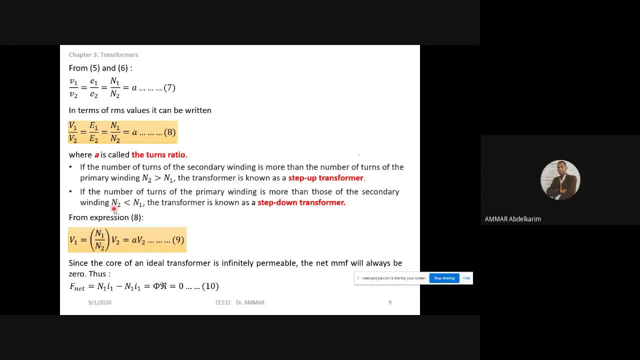 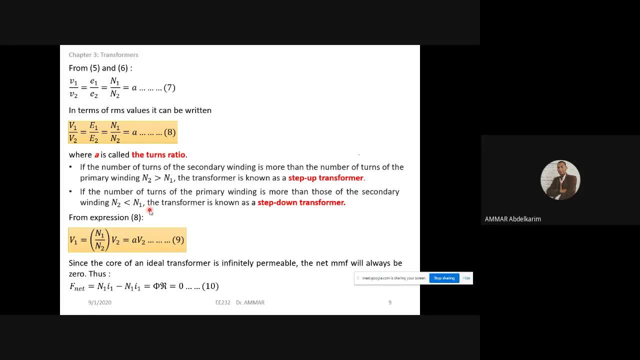 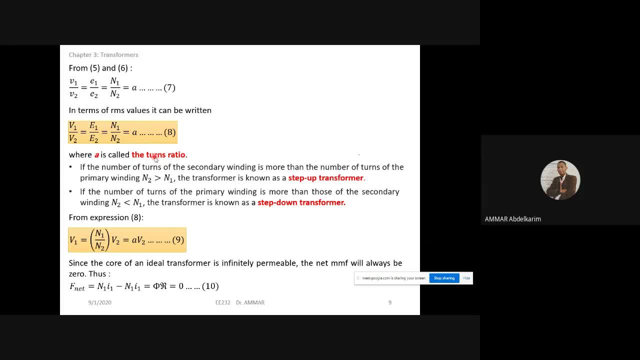 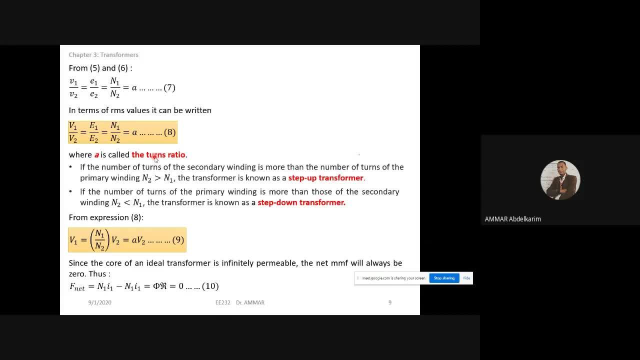 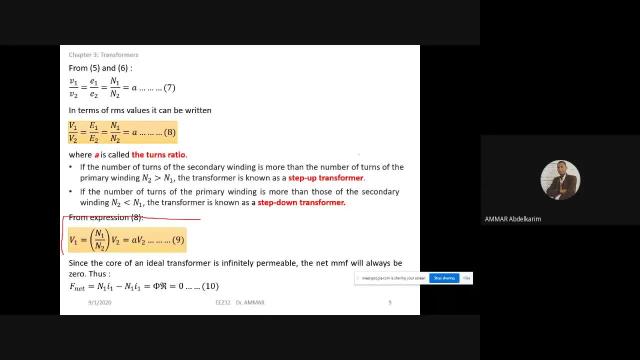 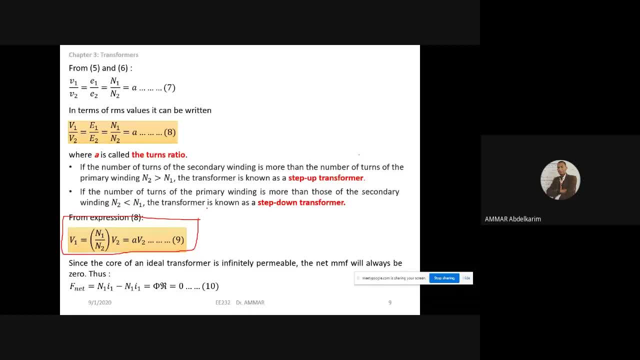 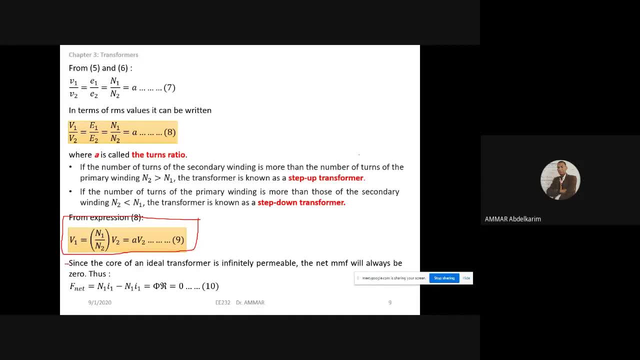 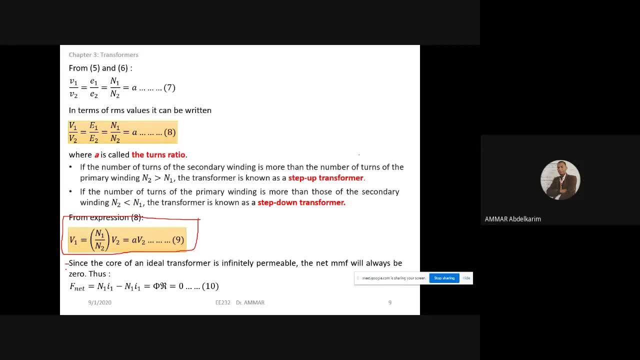 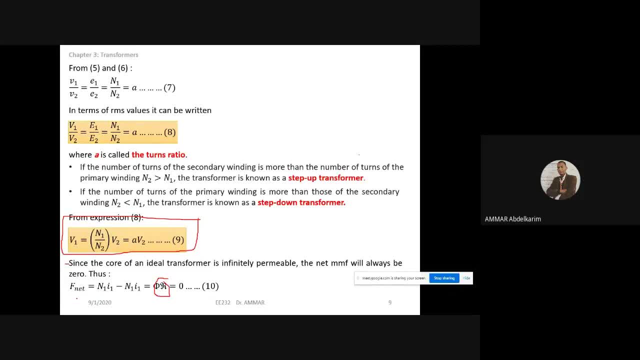 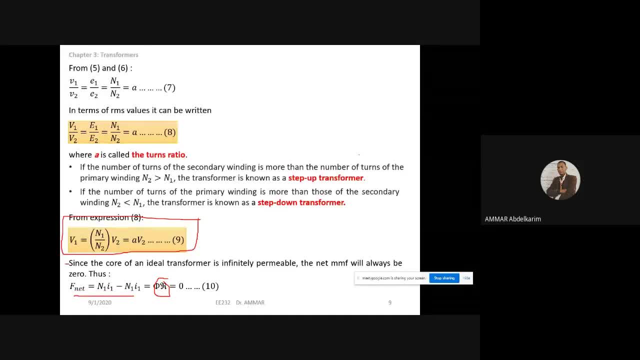 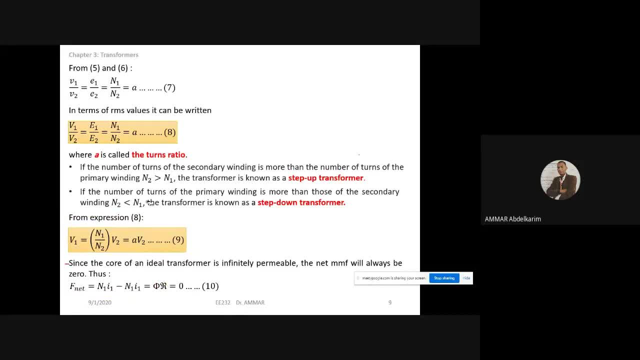 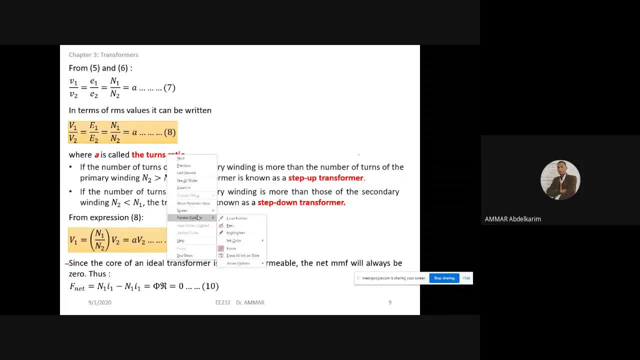 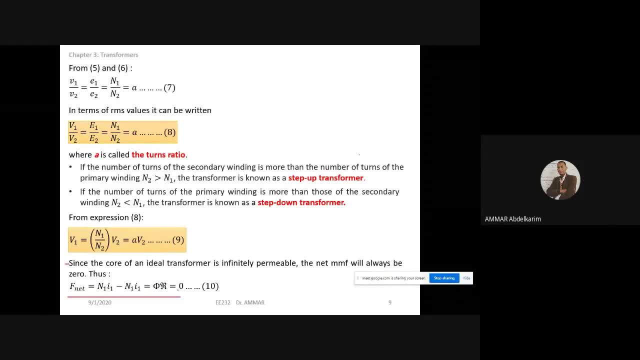 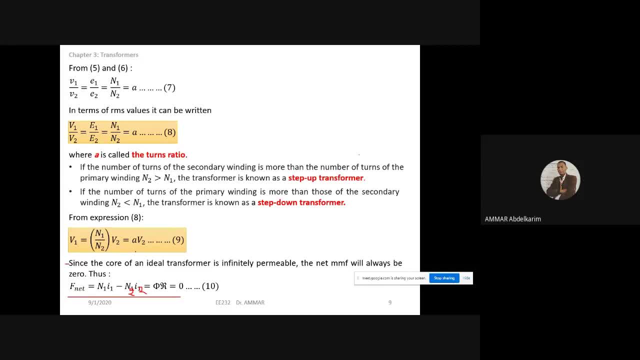 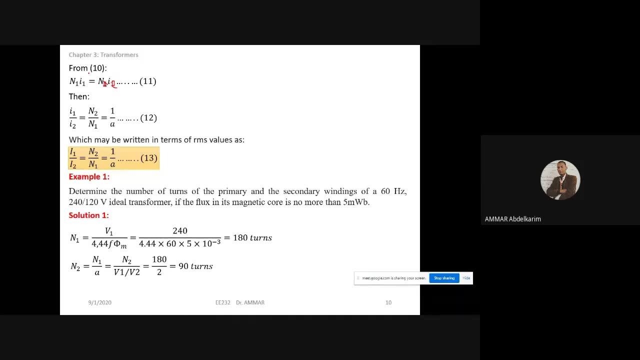 Okay, Let's take the simplest example we can, Because the reluctance is 0, the permeability is infinite. Using this expression – okay, the mistake here. also, I should correct it From 10, we have nn1 times I1 equals to n2 times I2.. 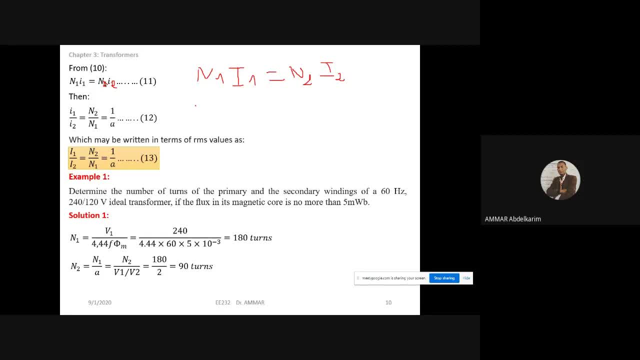 Then, according to this expression – according to this expression, I1 over I2 equals to what Equals to nn1.. Okay, To n2 over n1.. So here it's vice versa with voltage. Okay, We have written on the table before. 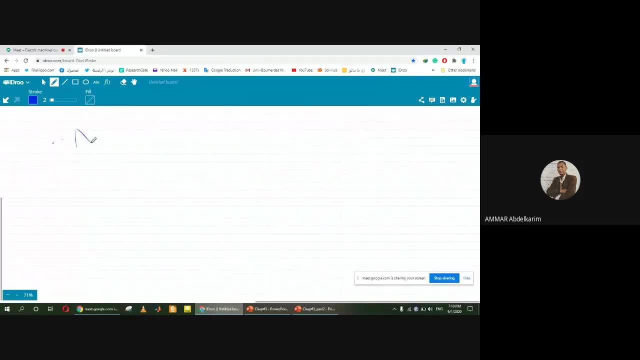 We have written n1 over n2 equals to E1 over E2 – sorry, E1 over E2 equals to V1.. Okay, We have written on the table before. We have written on the table before Over V2.. But it's equals to I2 over I1.. 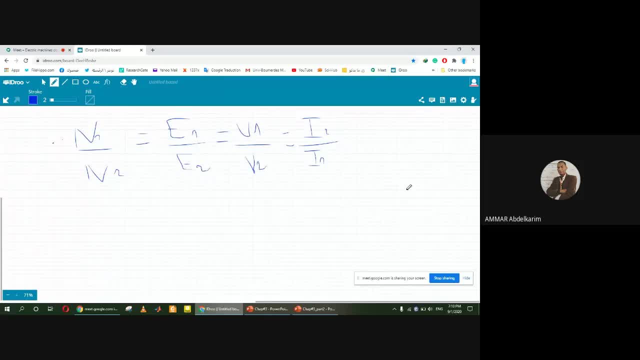 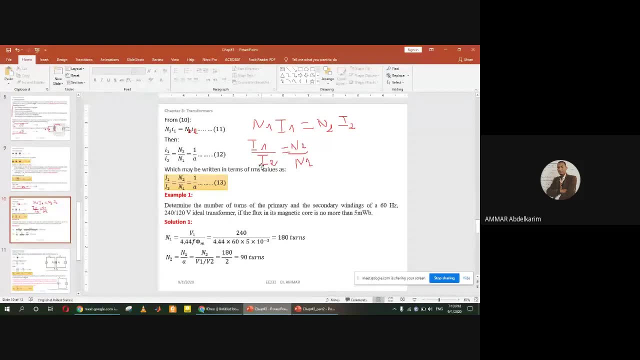 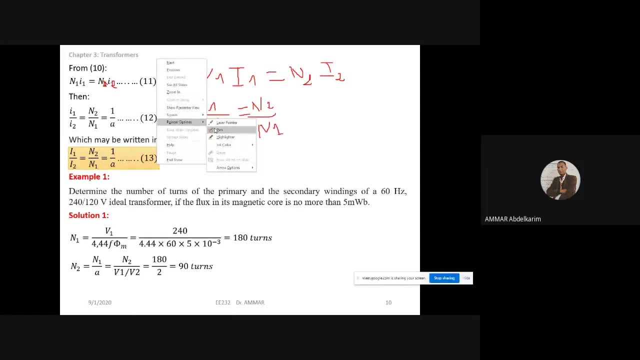 Okay, So it's vice versa between voltage and the current, the relationship with the turn ratio. Okay, So I am using the expression of the MMF: n1 times I1 equals to n2. times N2.. Then I1 over I2 equals to N2 over N1.. N equals to 1 over A. This one is the. 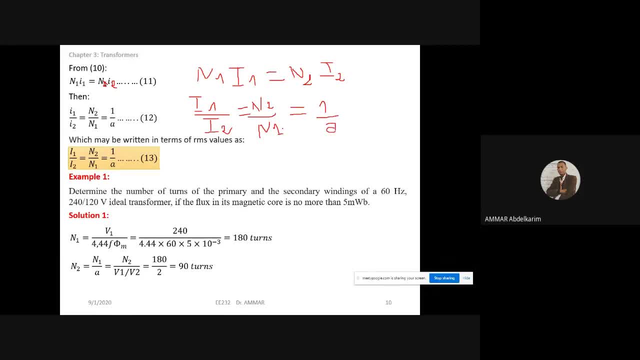 1 over A. So the relationship between the terms ratio, the term ratio, the relationship of the term ratio with voltage and the current is opposite. Okay, that's why when we said step-up transformer, it increases the voltage but in the same time it decreases the current. 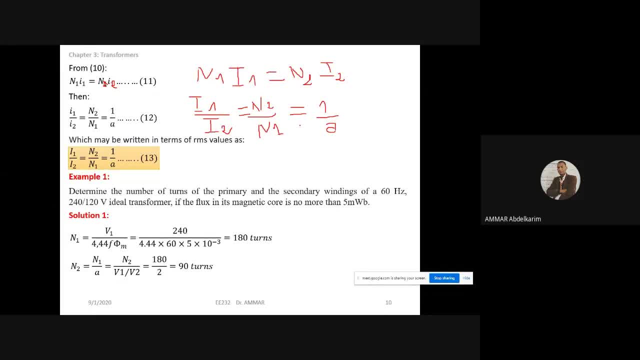 Also the step-down transformer. it decreases the voltage but increases the current. You know that the transformer does not change the power. The power S, for example, of the primary equals to S of the secondary, the apparent power, So, which means that V1 times. 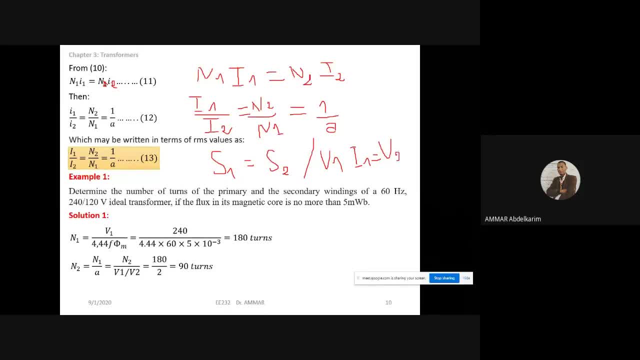 I1 equals to N2 over N2.. Of course, with losses here in ideal case. Okay, So the power does not change, They change the voltage and the current, but this product stays the same. Okay, So the current when? 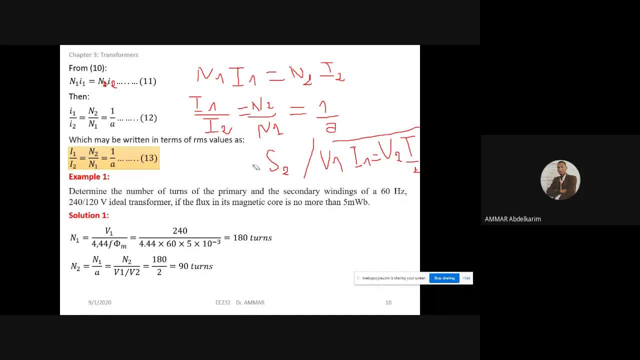 it's step-up, it always. We talk about voltage. Okay, We talk about voltage, It's step-up. It increases voltage but in the same time it decreases the current. Same thing with the step-down: It decreases the voltage and in the same time. 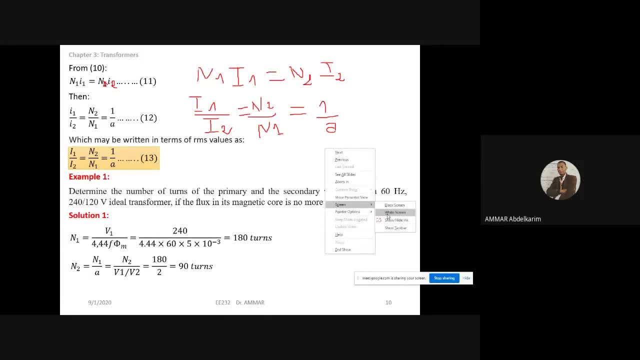 increases the current. Here we have an example. We have an example. Okay, Is it clear here with the current, before seeing the example: Yes, Yes, Yes, Yes, Okay. So it's the vice versa As the expression we have written here in the table. Okay. 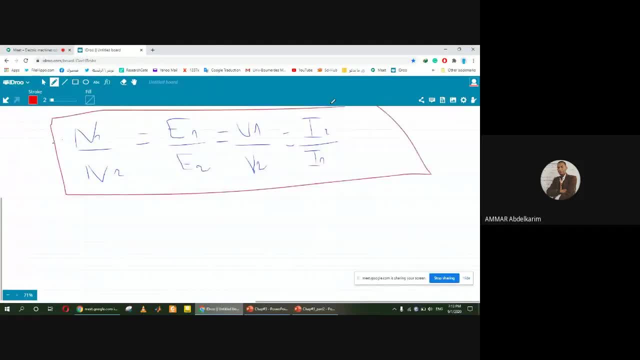 So N1 over N2, which is A equals to E1 over E2, equals to V1 over V2, but it's equal to I2 over I1.. So it's opposite with the current. That's why we have that. 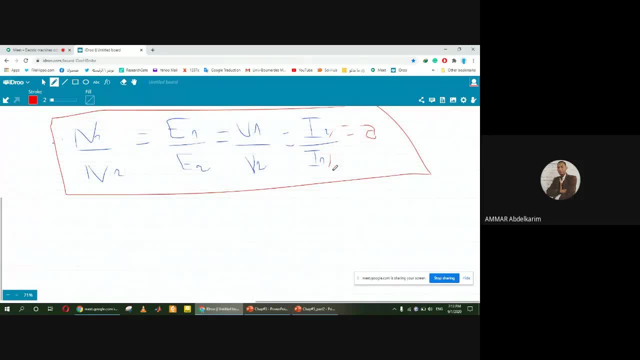 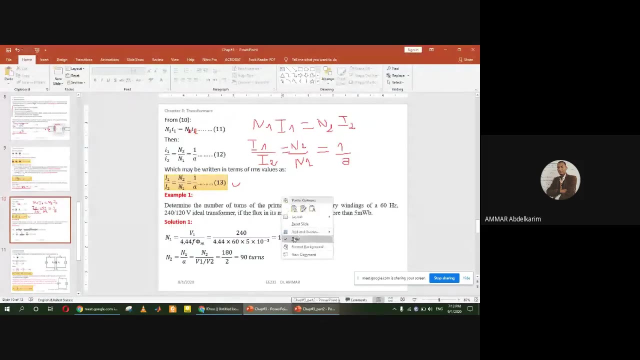 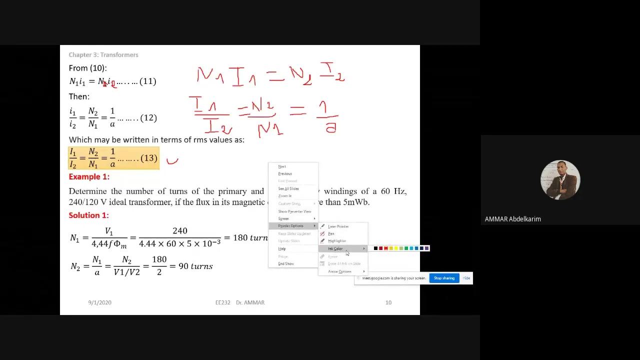 Yes, Yes, we said that the the operation of the transformer: okay, when it increases the voltage, it decreases the current, and when it decreases the voltage, it increases the current. okay, let's see this example. it's a simple one. okay, the eraser- where is the eraser? okay, no, there is much. okay, determine the number of terms of the primary. 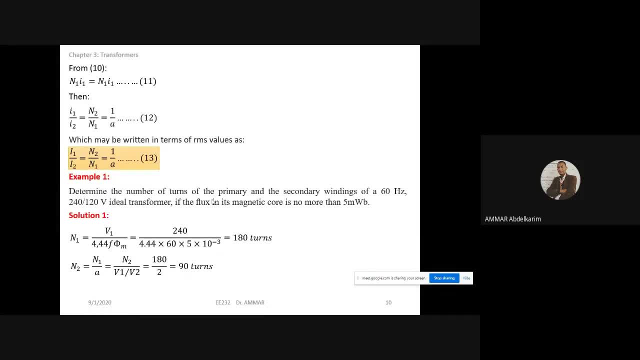 and the secondary winding of 60 Hertz, 20 to 240 and 120 ideal transformer. so when we, when we, when we write like this, so this is the high voltage and this is the low voltage if the flux in the magnetic core is no more than 5 milli, wherever, okay. so using the 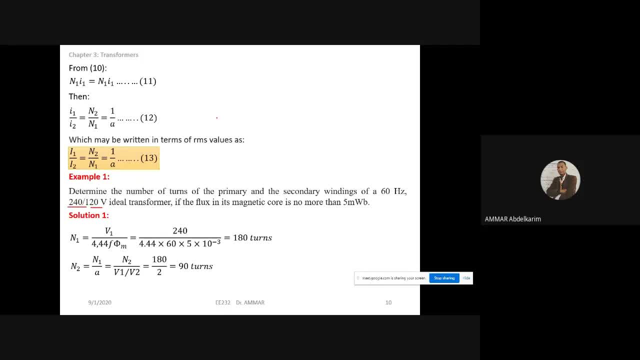 expression of. we said what we said when we explained the principle of operation of the transformer. so if this is the core, so if this is the core, we said that the voltage of the transformer will decrease. the current and the primary voltage of the primary will create a flux here, then this flux will create a voltage. 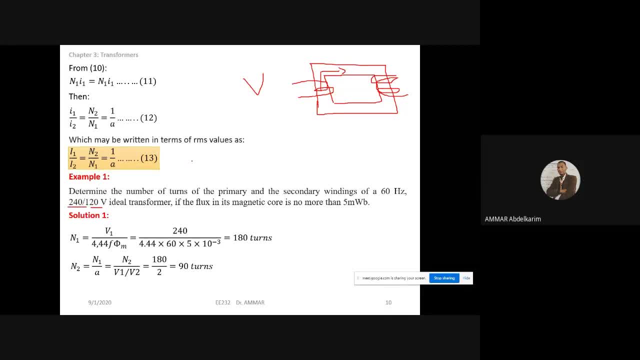 in the secondary. So, using Faraday's loop, the expression of the voltage V1 equals to what Equals to 444 times n, times f, times phi max. So here we have n1, we have the frequency. frequency, of course, is the same. 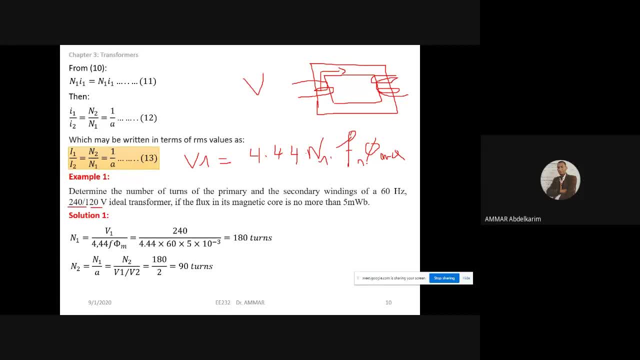 The transformer always keeps the same frequency and almost the same power, if we not consider the losses. okay, And phi max. So using this expression, n1 equals to what Equals to V1 over 4.44 f times phi max. 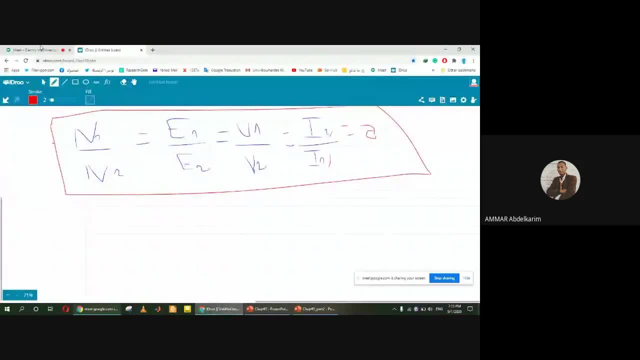 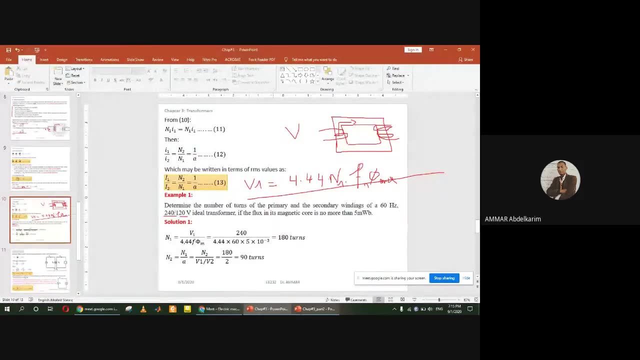 Okay, Okay. And this equals to what? Okay, This equals to what. This equals 240 over 4.44 times 60 times 5 to the power minus 3, because it's milli Weber And the number of terms is 140.. 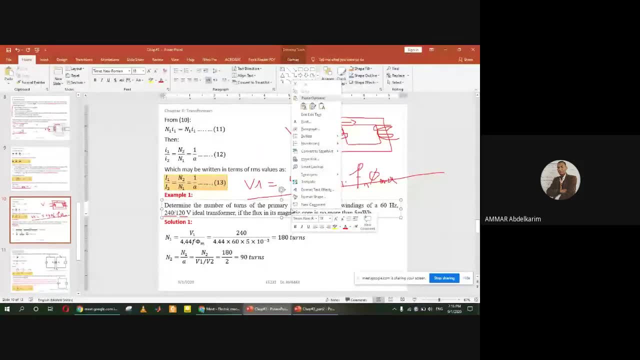 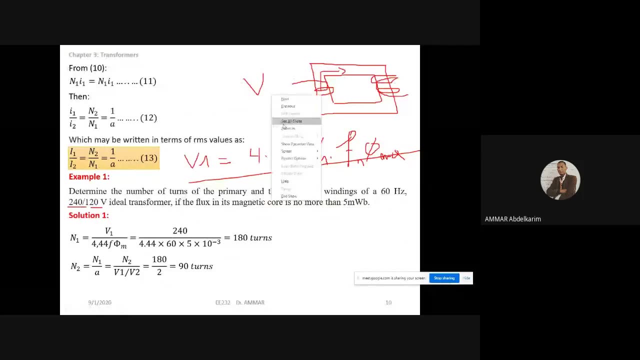 Okay, 180.. Okay, 180.. Now this is the number of terms of the primary. Okay, we have found it using Faraday's law. So now how we can find the secondary. Of course, using the expression of the term ratio, we have n1 over. n2 equals to V1 over. 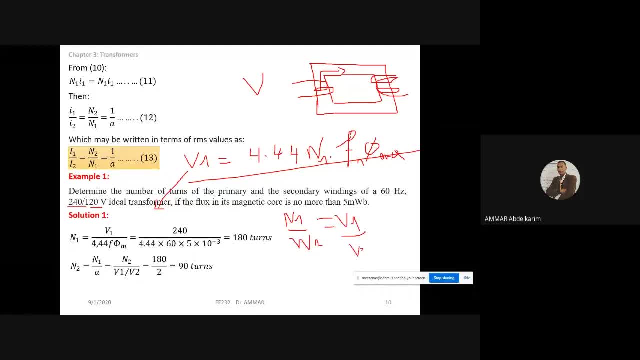 n2.. Okay, V1 over V2.. We have V1 and we have V2, of course, V1 is 240 over 120, which is equals to 2.. Be careful: This expression is for the ideal transformer, not for the real transformer. 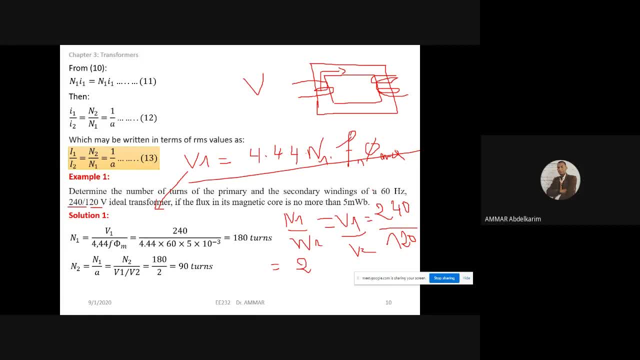 Okay, It can be valuable for the real transformer in one case, When, In the no-load case, If the transformer is not connected the real transformer, if it's not connected to the load, there is no resistance. The current is almost zero. 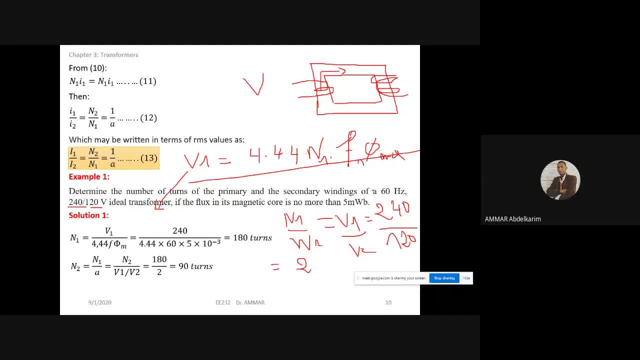 So this expression can be valuable in one case when we don't have load in the real transformer. But this expression is exactly for the ideal transformer. So n1 over n2 equals to 2, which means that n2 equals to n1 over n2.. 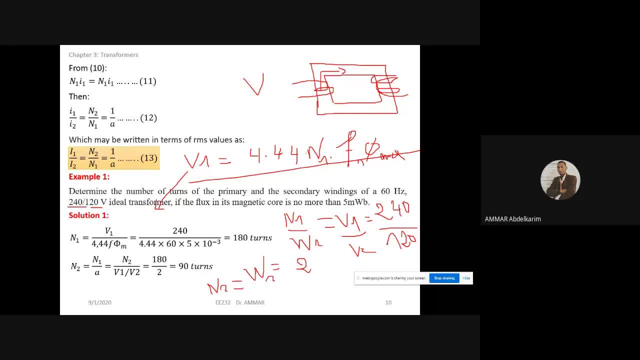 Okay, And it's 990 turns. Yes, Sir, I have a question concerning this exercise, Concerning n2, can we use the same expression? Then, can we use the same expression: Calculate n1.. Yes, Can we use the same expression. 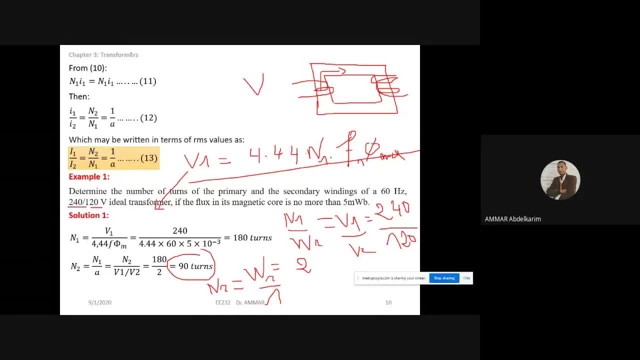 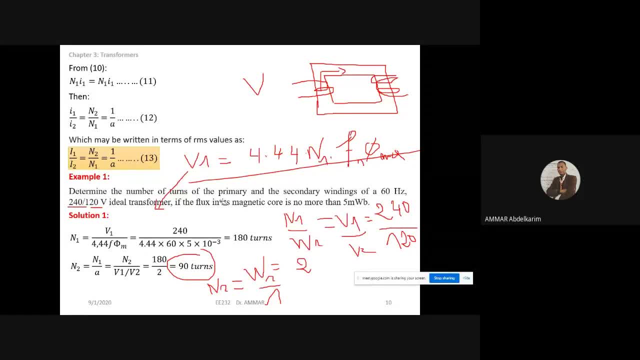 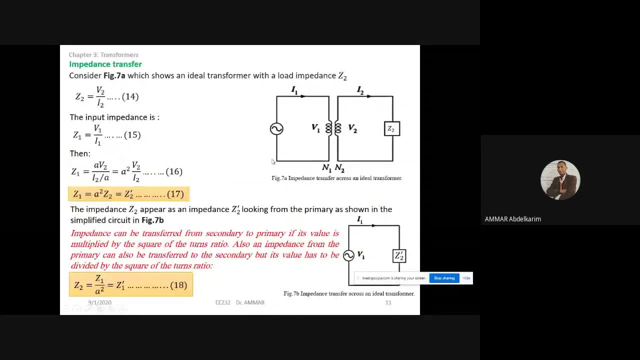 You will. The flux is the same, The frequency is the same. We are going to replace 240 with 120.. Okay, Yeah, So it's the half. Yeah, yeah, Yes, It's the half. Okay, So I should stop here. 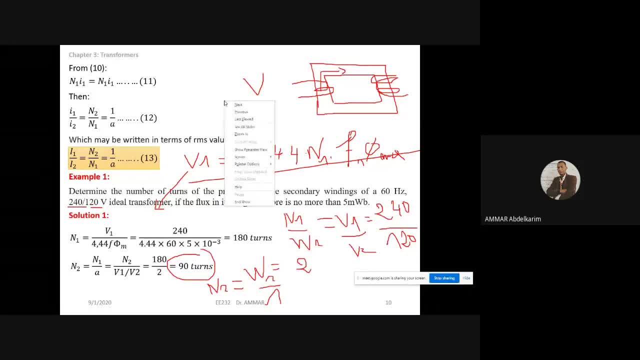 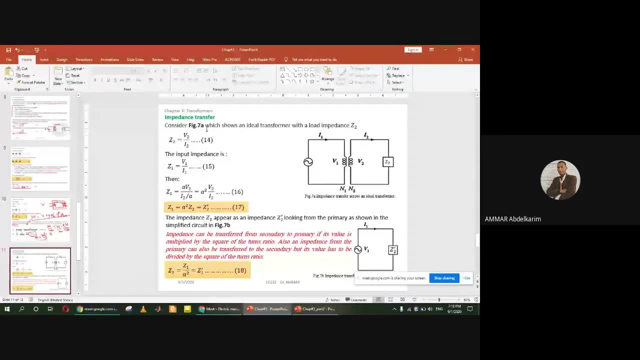 Create the new. Okay, We've done almost one hour. Okay, I should stop here. We still have impedance transfer: one element, Then we pass to the re-transformer. Okay, 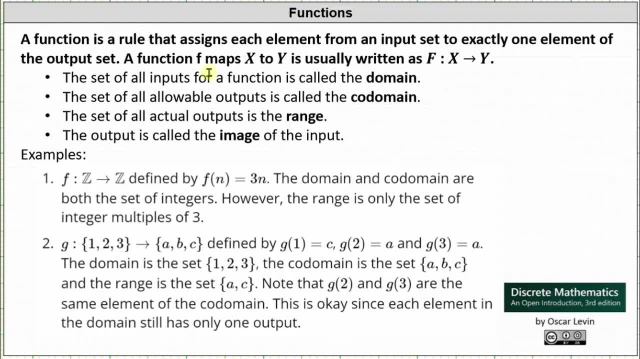 Welcome to an introductory lesson on functions. A function is a rule that assigns each element from an input set to exactly one element of the output set. A function- f maps x to y- is normally written using the notation shown here, where we have f, colon, x, arrow, y, The 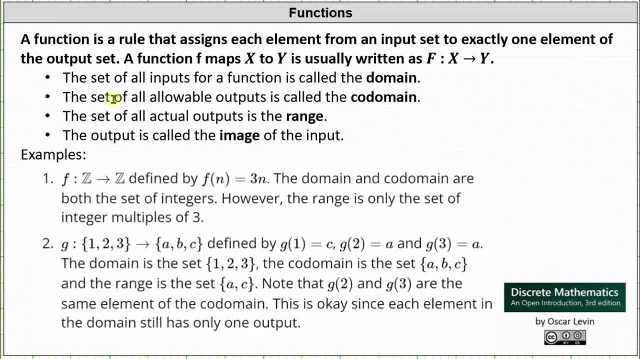 set of all inputs for a function is called the domain, The set of all allowable outputs is called the codomain And the set of all actual outputs is the range. In previous math classes you may not have referred to codomain, but there is a difference between the codomain and range. Again, 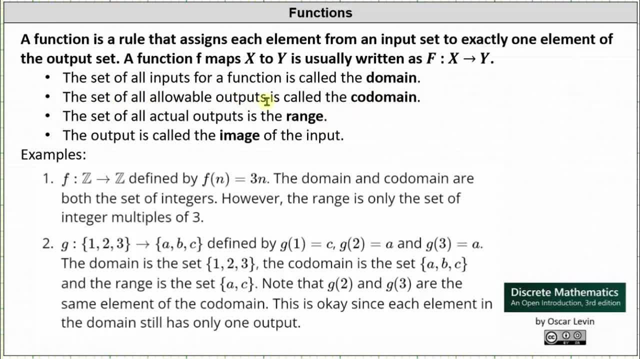 the codomain is the set of all allowable outputs, while the range is a set of all actual outputs And the output is called the image of the input. Let's look at some examples of functions. Number one: we have the function f, which maps the set of integers to. 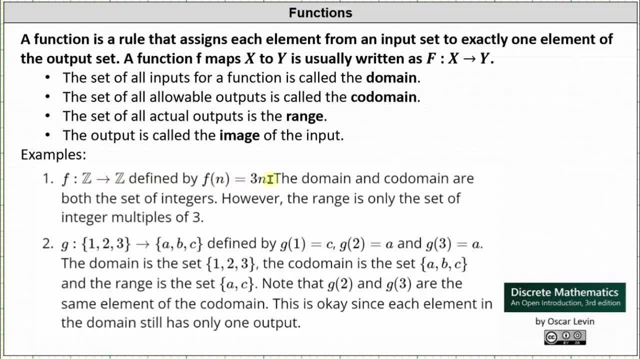 the set of integers defined by f of n equals 3n. The domain indicated by the first z and the codomain indicated by the second z are both the set of integers. However, the range is only the set of integer multiples of three. This is because the function is defined by f of n equals 3n. So 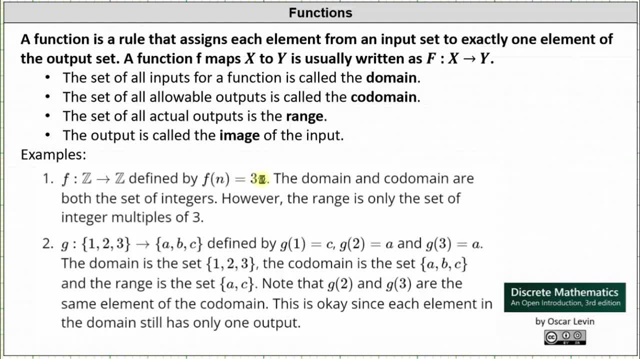 while n can be any integer, notice the output is always going to be three times an integer, giving us a range of the set of integers. So again, notice how the codomain and range are different in this case. Next we have the function g that maps the set containing the elements of 1,, 2, and 3.